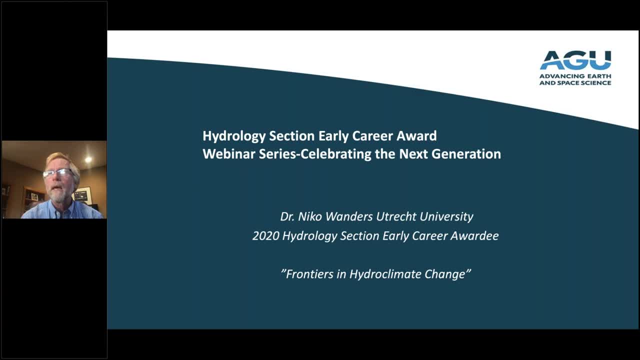 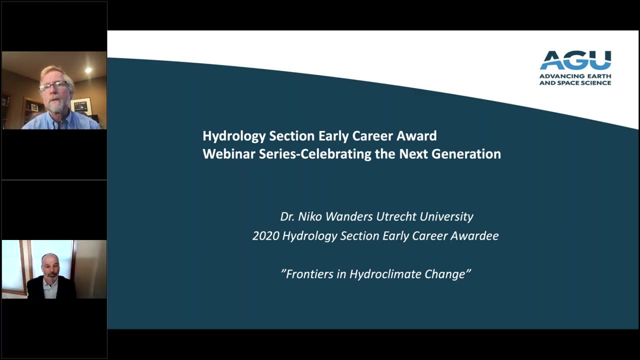 see me at the end. We have a few announcements for the fall meeting and I will catch you at the end of the seminar. It's now my pleasure to introduce Dr Reid Maxwell from Princeton University. to introduce the speaker, our awardee winner this week, Dr Nico Wanders, Reid Hi. Thanks so much, Scott. 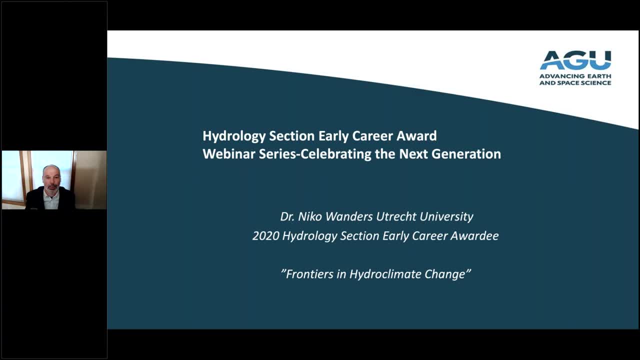 It's with really great pleasure that I introduce Nico Dr Nico Wanders, who's assistant professor in geosciences at Utrecht University- Everybody who's Dutch just cringed- As one of the 2020 AGU early career hydrologic. 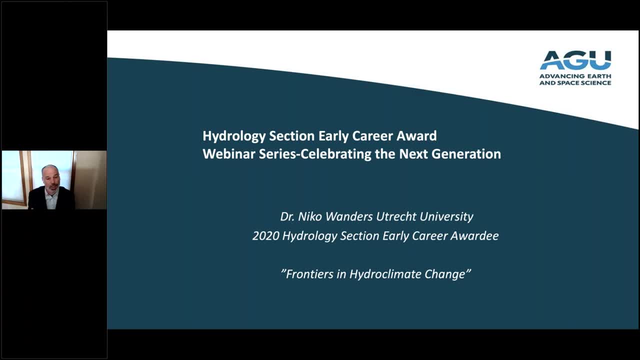 sciences early career award recipients and our third speaker in this amazing seminar series today. Just a quick introduction: Dr Wanders has made really impressive contributions in four areas: Understanding drought and its feedback on human water use. hydrologic modeling and forecasting hydrologic impacts of. 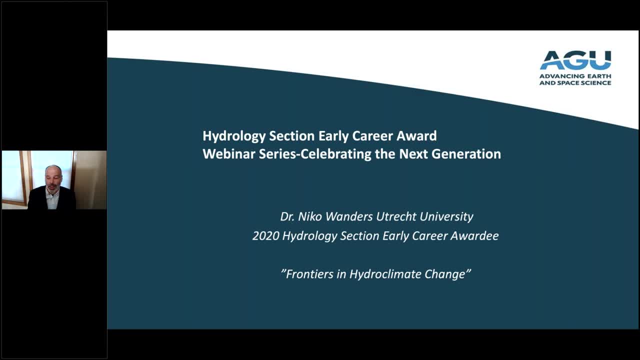 climate change and hydrologic remote sensing. Wanders research is at the forefront of understanding the large-scale relationships between hydrologic extremes and hydrologic models, And he's also been a member of the National Institute for Climate Change and Human Water Use, which is exactly what you're going to hear about today. 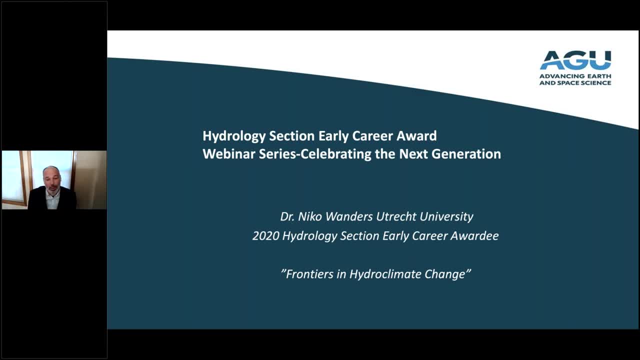 Dr Wanders has won numerous awards. However, I'm not going to spoil the citation. You're going to have to tune in during the AGU awards ceremony to hear more. For now, let's all give a virtual round of applause and welcome Dr. 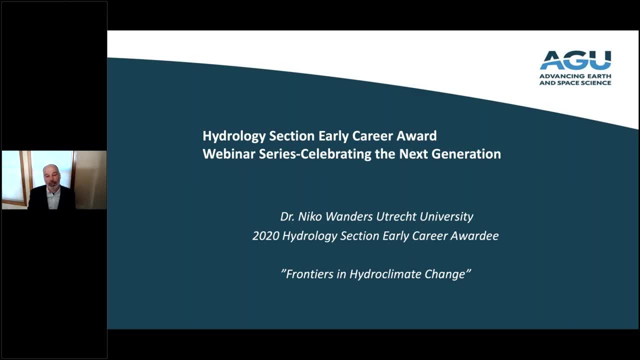 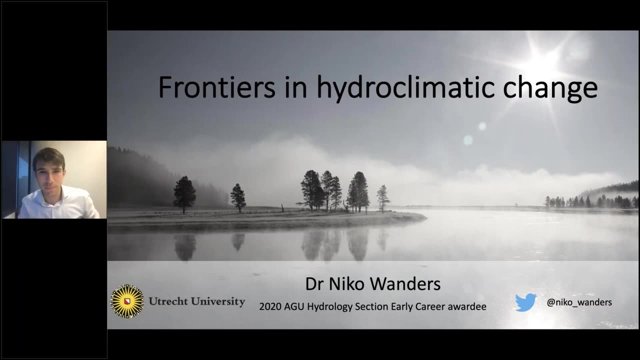 Wanders' lecture on Frontiers in Hydroclimate Change. Thanks, Reid, Thanks And welcome to you all to my lecture, Frontiers in Hydroclimatic Change. I want to start by thanking some people who have been very important for my career. 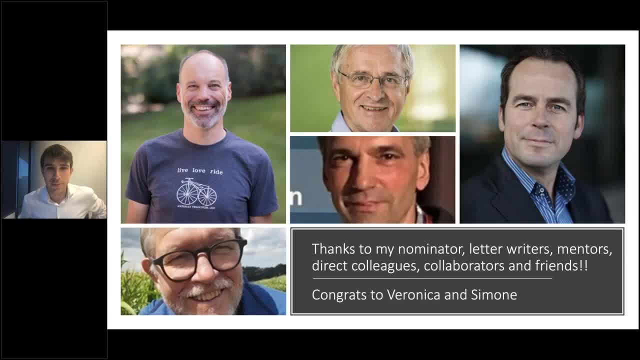 Of course, my nominator, Dr Reid Maxwell, who just gave me a very nice citation, Some of the letter writers, Dennis Lettermeijer, Martin Clark and Lennart Alexson, who supported the nomination, And, of course, some mentors I've had along. 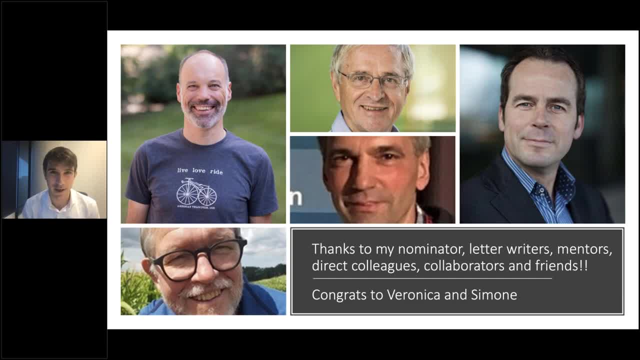 the way: Hennie van Laanen from Wageningen University, bottom left, Erik Wood, Princeton University, and Mark Bierkes on the top right, who's now also one of my mentors here in Utrecht, and Stephen Young, who's in the center of the picture, who actually gave me a PhD in, although 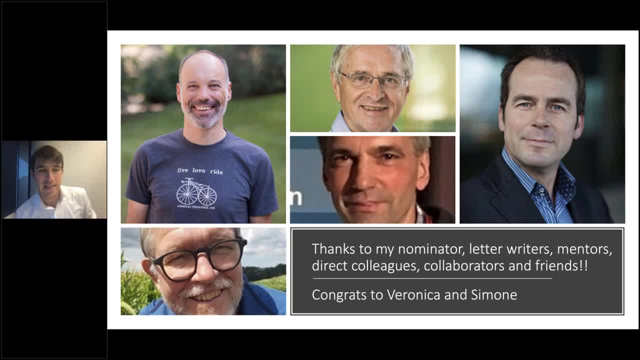 we're talking today about droughts, where he gave me a PhD in floods. So, and of course, I want to congratulate Veronica and Simone. I also like to thank my family, who's not only supported the work I do, but also deal. 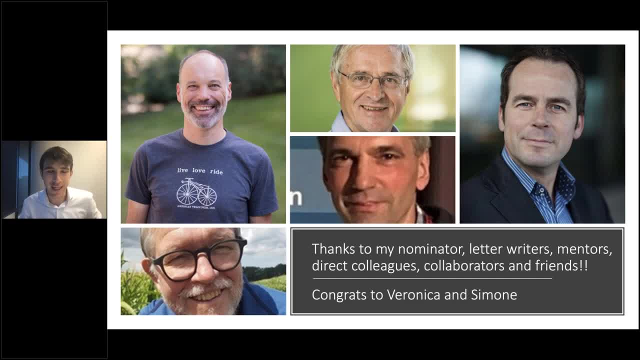 with my daily fascination for hydrology and droughts, And I think one of the you know signs how we can see this is by the disturbing amount of pictures with water related items I have for my holidays. So I also would like to thank them and for taking me outside as 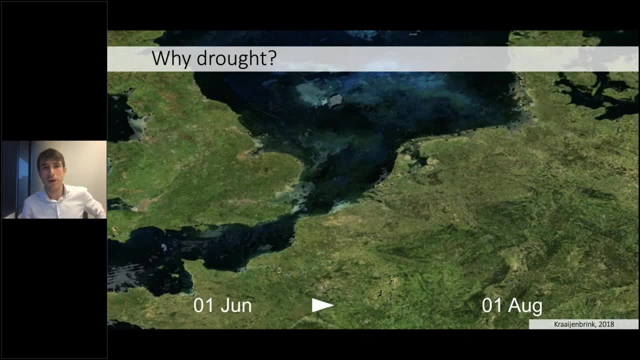 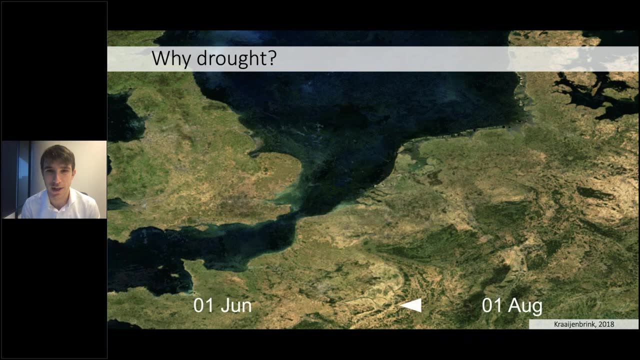 well for my parents. So you come from the Netherlands. why do you study droughts? I mean, it's the country known by for floods. Actually, we had a couple of big droughts running 2018, 19 and 20.. Here 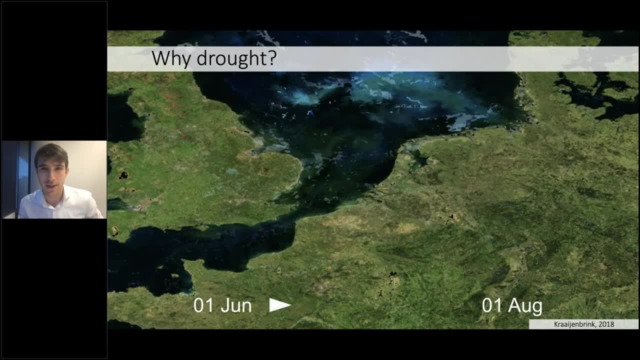 I have an animation of Philip Kruijbrink, who's a postdoc here in Utrecht, showing the impacts of droughts, And what fascinates me here is that it's kind of a large scale phenomenon. It's not like 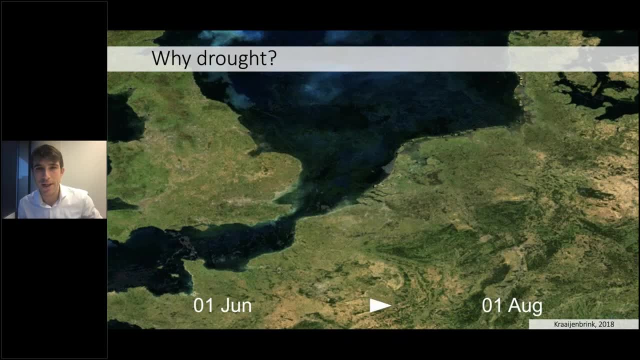 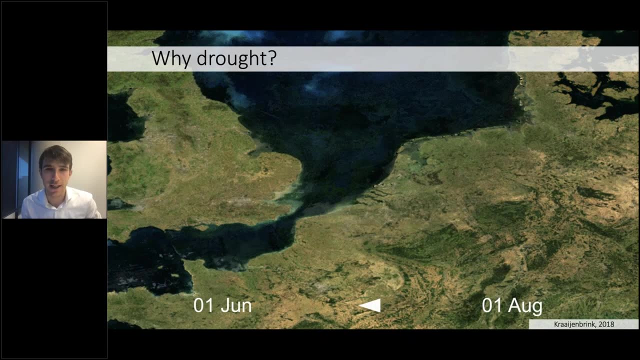 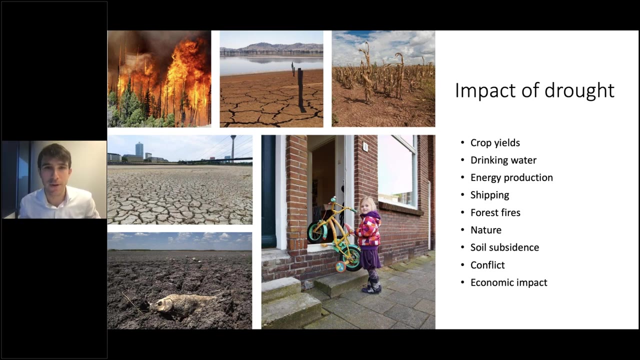 one location you see in Northern France, the UK, but even in the Netherlands you see yellow vegetation popping up. So even a country like the Netherlands is hit and some of the impacts that we have, for example, or globally have, is basically loss in crop yields problems. 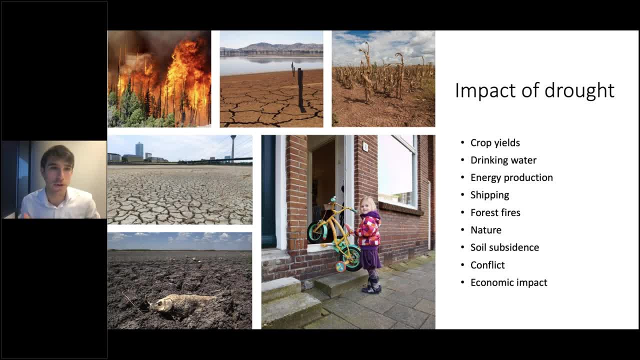 with drinking water supply, energy production. of course, shipping- when there's no water, shipping is going to be very difficult- forest fires. So these are the different types of problems. So, in terms of the droughts, the most important one is the climate model. So there are all. 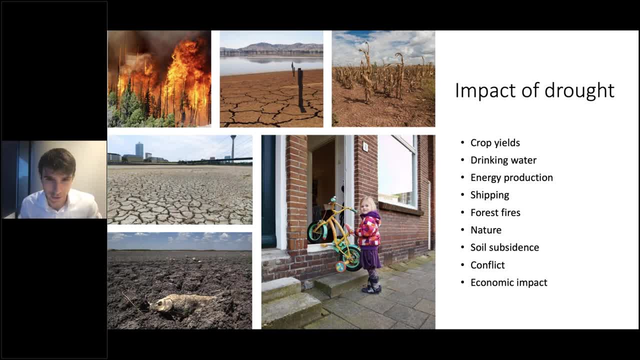 really three types of droughts- and this is just sort of a little summary- to the performance of climate models. So we have droughts where the climate models are very much in conflict with the climate models. So I'm going to just quickly talk about the two types of droughts. 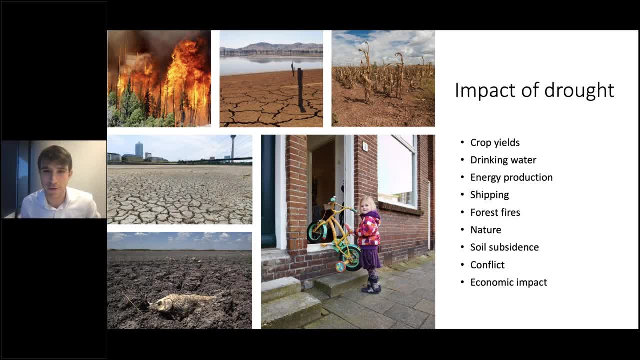 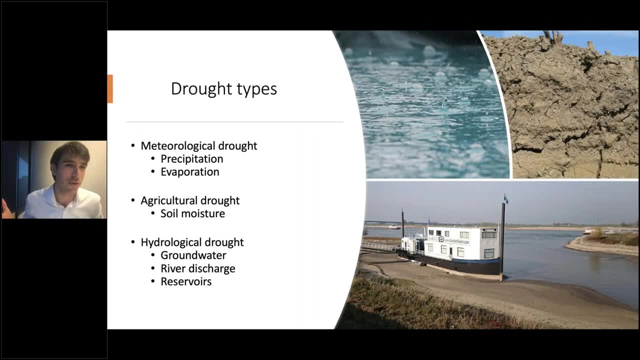 The first is, of course, one that I mentioned. the droughts are when there are polluted fields, when there areна lot of people on the roads at very light speed. That's a good one, Yeah. types meteorological drought basically caused by precipitation and evaporation. agricultural. 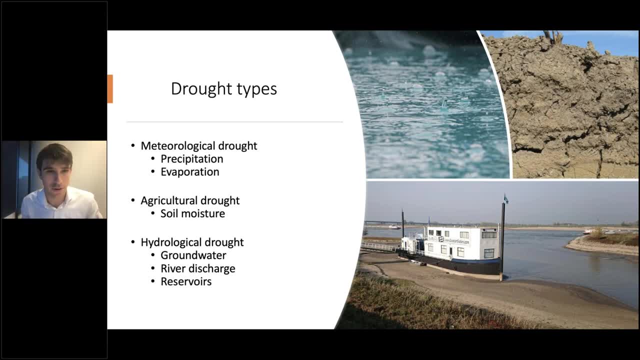 drought, soil moisture and then hydrological drought. that's the one I focus on most frequently impacting components like groundwater, river discharge and reservoirs. And drought is not something just of the last 20 years. Actually, I have here this paper. 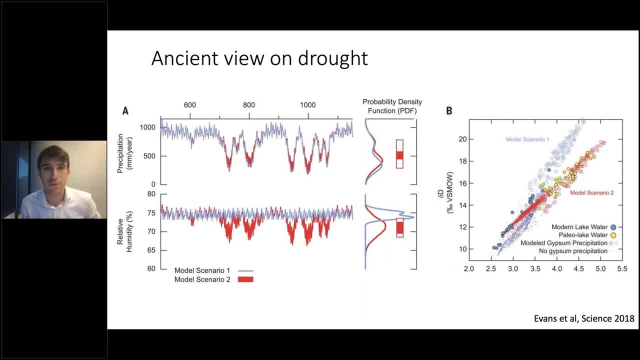 by Evans et al from science, and they actually used lake deposits to indicate, for example, how the Maya civilization was affected by droughts And whether or not it caused their collapse. that's still up for debate, but at least you see that droughts have already. 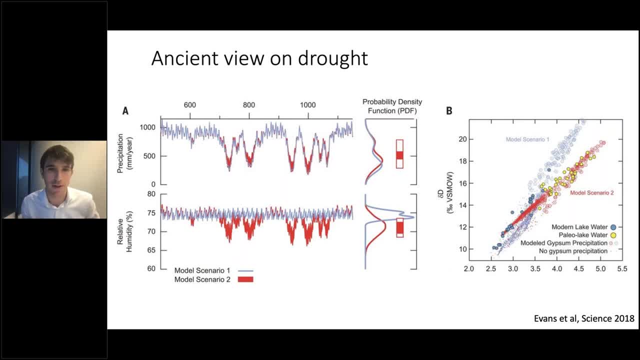 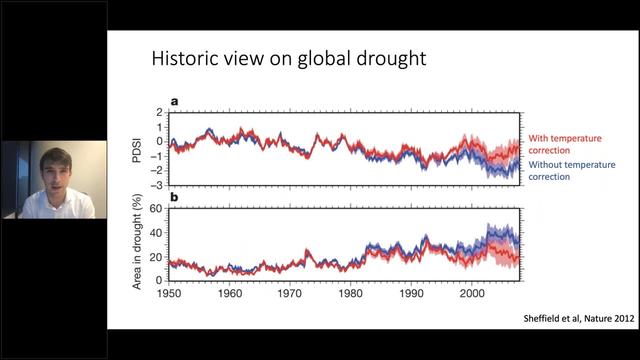 quite a historic impact. But for this lecture, we'll focus more on the current and the future, but I wanted to show that it's not just something that's happening now thanks to climate change. I want to start by with this graph by Justin Sheffield from Nature in 2012.. Actually, before. 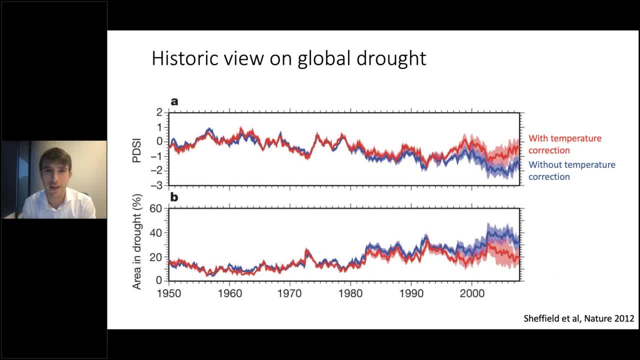 I got to Princeton they published this and it shows very nicely the development of global droughts around the world. And he showed, together with Eric, that it's important to also look at the impact of temperature when you're doing your evaporation calculations. 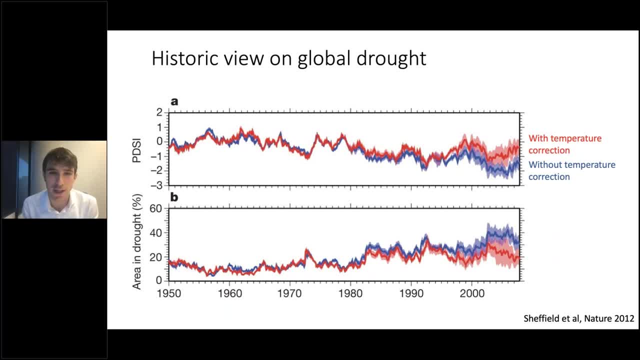 So we often we have this problem with droughts that we try to relate them to the past, but we also have an ongoing trend on top of that. So you see, here, here on the the top, the pdsi is the former drought severity index, a frequently used drought indicator. 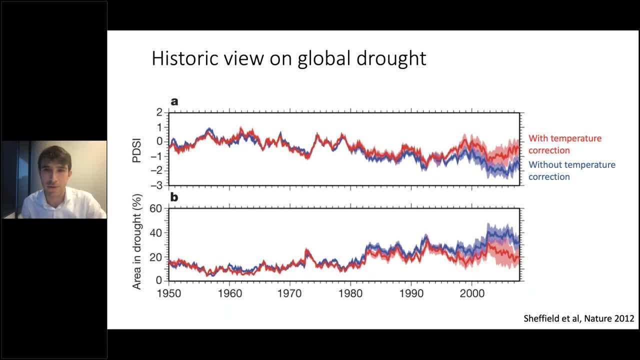 a zero is average and everything in the negative is a drought condition. you see the global average and you see, without the temperature correction that's the blue line. you see severe droughts everywhere past 2000 on the on average on the globe. but if you take into account temperature, 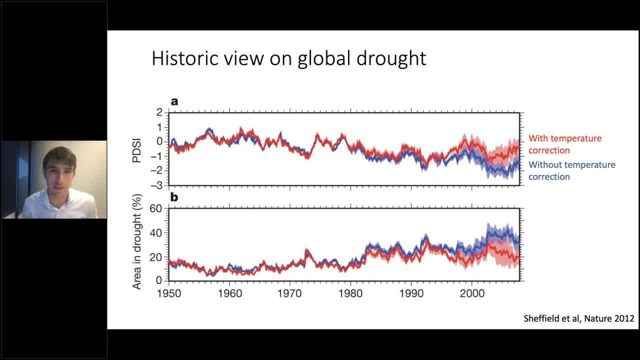 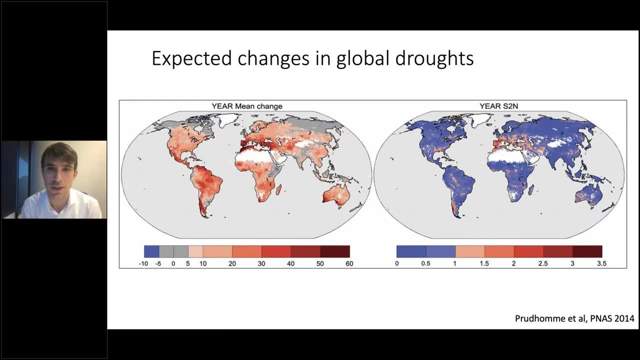 correction. actually, the impact is significantly less. the temperature impact will also impact the evaporation in the future. so here i uh. let's show you a paper by prudhomme in plus 2015-14 from the easymet data, which is a large ensemble of hydrological models that has been used in 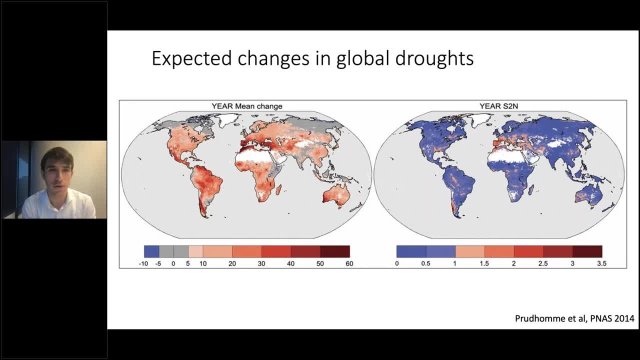 combination with climate models to generate future outlooks of droughts but also floods. but of course, we focus here a little bit on the droughts and you see some hot spot areas that pop up very frequently, like the mediterranean, and also south south america, southern south america. 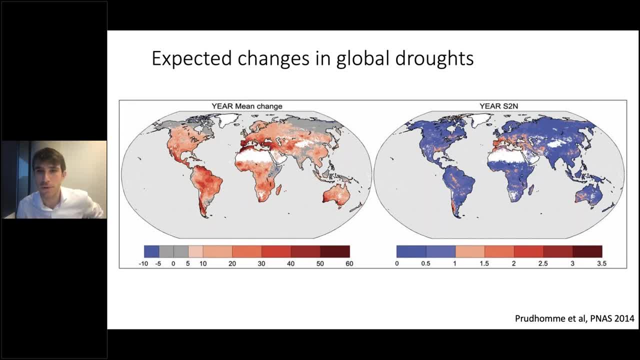 um, so, and they actually show that there's also a signal to noise. that's the picture on the right and that's for the red regions. you can actually say that the signal to noises is very good and that you have a very clear indication of where things are heading, and this is 2014 and this field. 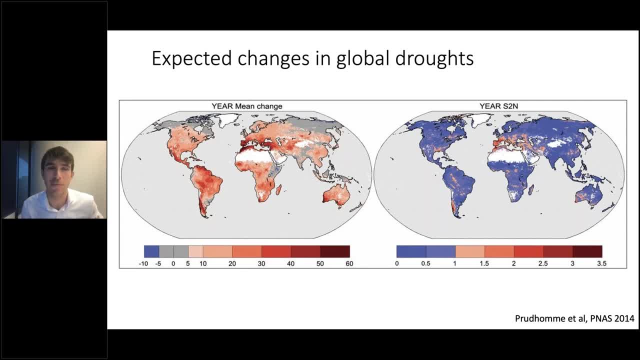 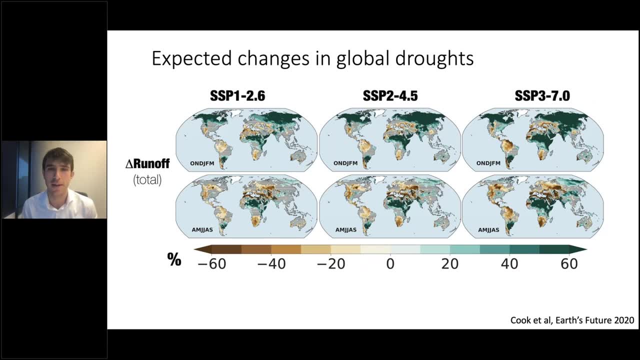 is moving rapidly. i mean, we've been six years past the study and there's more and more have been done. for example, we now have the new c-mip6 simulations, which provide more higher resolution, more accurate. this is a very important data that we are using here in this case, and we're using this. 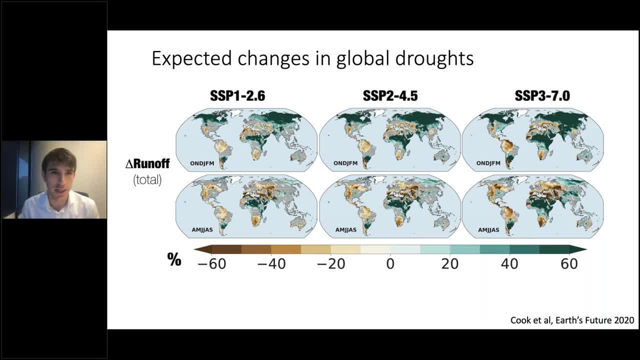 data on that we can use for climate projections on droughts. here i have a paper from earth future from 2020, by cook at all, and it basically shows a similar pattern and at the top you see the winter on the northern hemisphere and on the bottom you see the summer on the northern hemisphere. 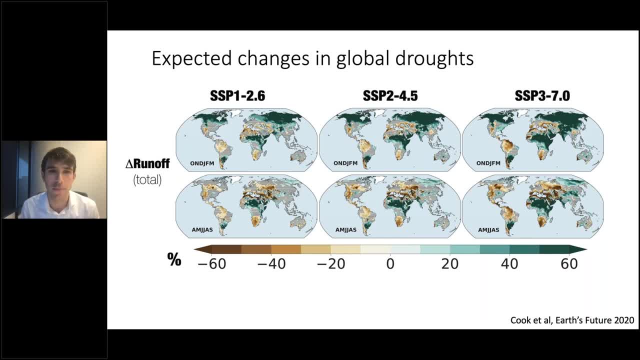 and you see also for arctic regions here that actually runoff in summer is going to increase. uh, at least if you believe the models. if you go from left to right you see more and more severe be conditioned, so warmer and more impacted. so in the arctic you have melt and that's most often. 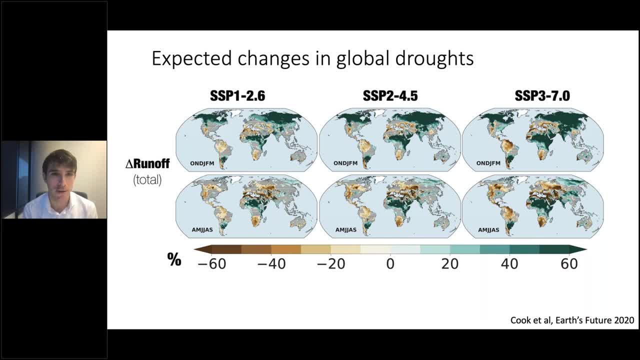 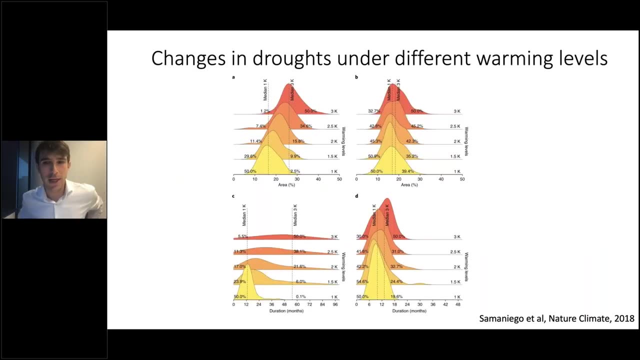 it's a melt of permafrost or snow or earlier melt of that, and then in summer, if you look at the bottom row, you see again that patch in the mediterranean popping up like severe decreases in runoff which will have a significant impact. this was also largely shown by samaniego at all. 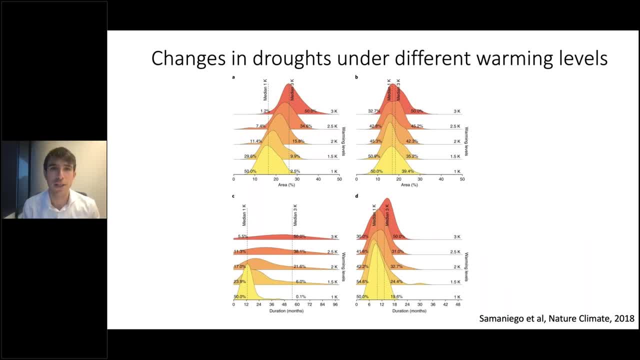 in nature climate chase in 2018, where they showed the changes in drought area on the different warming levels, looking at one, one and a half, two, two and a half and three decay k global warming and what you see is the area on drought on the top, uh, where you see on the left, top left and number a. 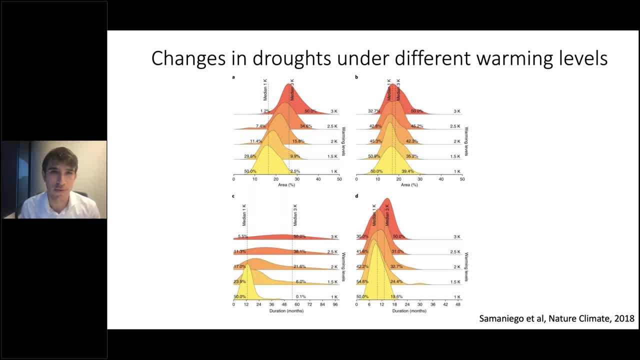 you see what? if we don't take into account changes, so you see 50 increase in that area. so that's quite a significant increase. if you do take into account that the norms and the climate is changing, then the impact is a little bit less. and you see the same for the durations that are, we get more, longer. 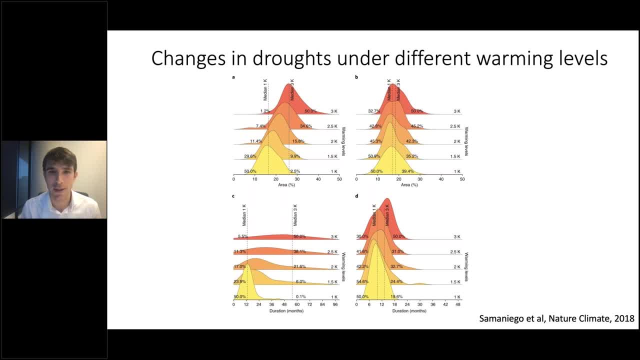 more severe droughts and um he, uh, they hypothesize that actually. uh, with this, climate change will also become a new norm, so the droughts that we think are heavy now will not be as heavy anymore in the future. we will just see them as a nice summer day, to put it bluntly. 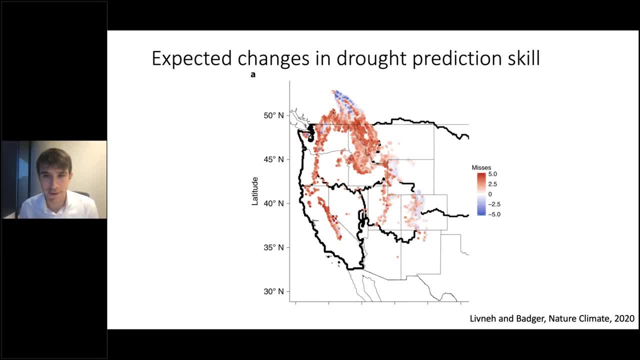 other aspects. this into a recent paper by uh, litany and badger in nature class in 2020, showed also that this- these expected changes in in droughts and climate change- will not only uh affect the drought itself and the runoff, but also the predictability, for example. 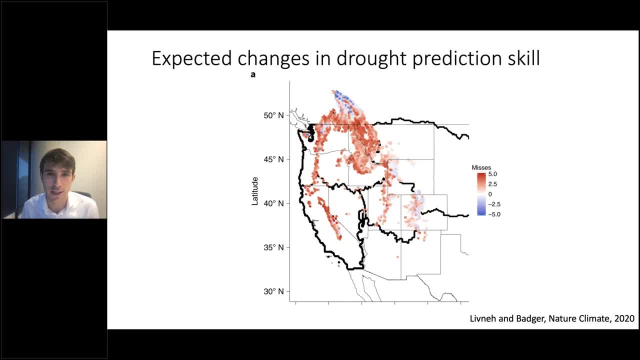 snow, droughts and winter discharge, or actually spring discharge, in this case only in all the red spots, you actually see that we have more difficulties trying to correctly predict those snow melt peaks, and that's also, of course, very important if you look at reservoir management, uh, and other water management issues. so that's that shows already quite some impact here in the 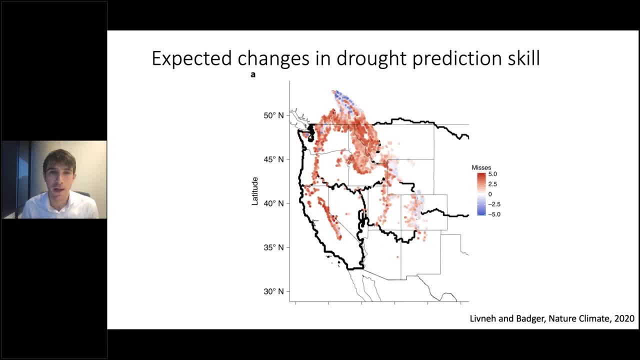 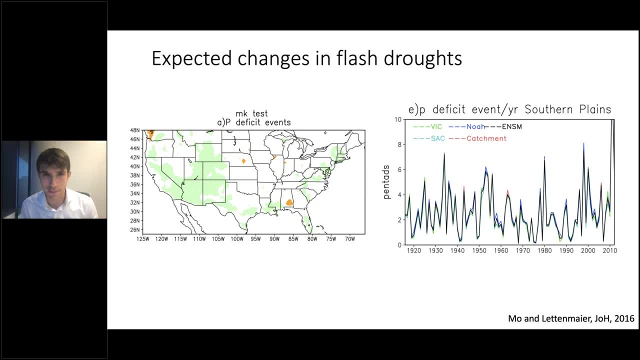 western us, for example. if we go then to the, the concept of flash droughts, which has been- uh yeah, identified in 2016 by mo and latimer and have been heavily studied since, we actually also see that those are increasing. so there's very rapid onset flash droughts that occur due to extreme meteorological conditions, and they're likely to be. 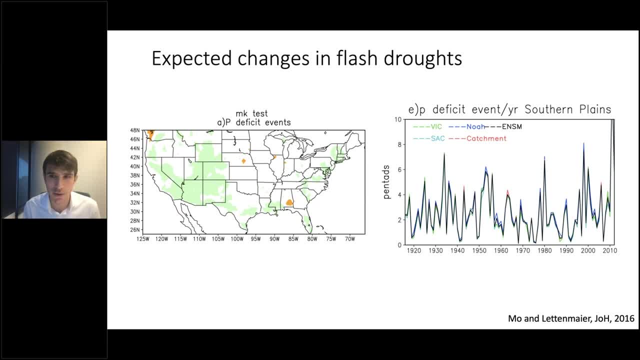 expected to increase um in the green areas over there you see the trend on the right for the historic period. you see spike towards 2011, but that's. i think we should just look at the general trends in that sense. but all these things and all these impacts are expected to change already from. 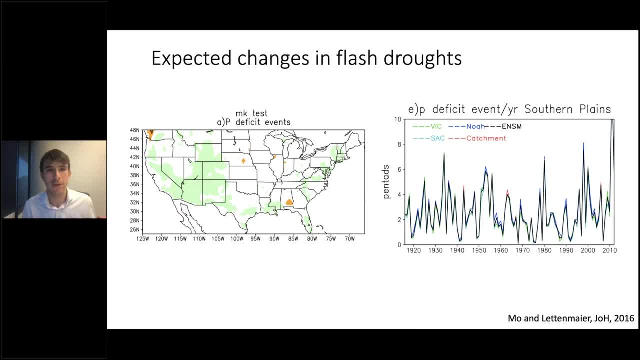 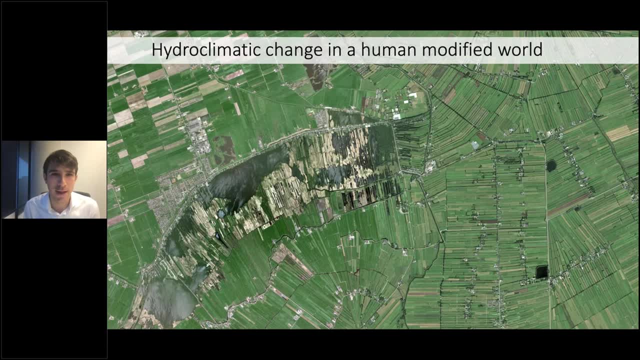 from what we have now. but i only talk here about, uh, natural and human natural conditions. but coming from a country that is basically man-made, uh, here you get a nice picture of what you can get when you land on the airport of amsterdam. um, you can actually see that nothing here is man or natural and everything is man-made. 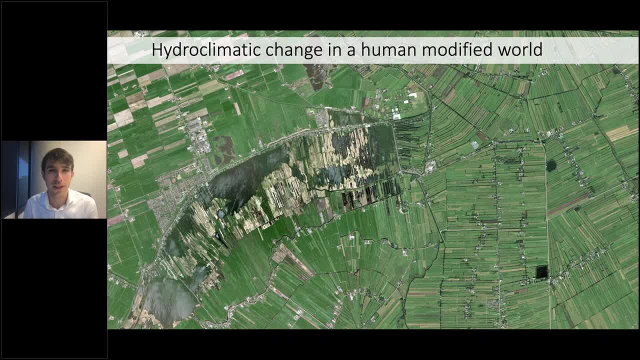 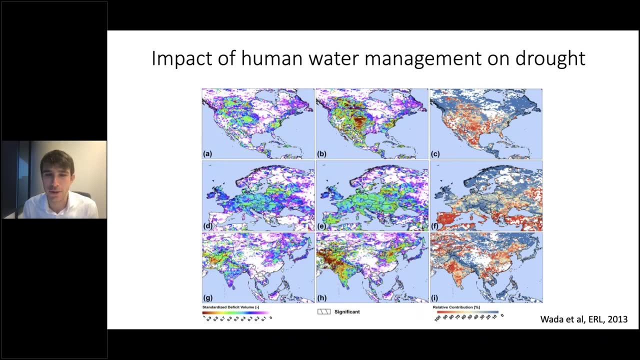 so if we want to study uh droughts in the future, we should actually take into account the human actions and the human impact. so here i show you uh a study we did, uh yoshivada and myself did in 2013, when we were both doing our phd as a 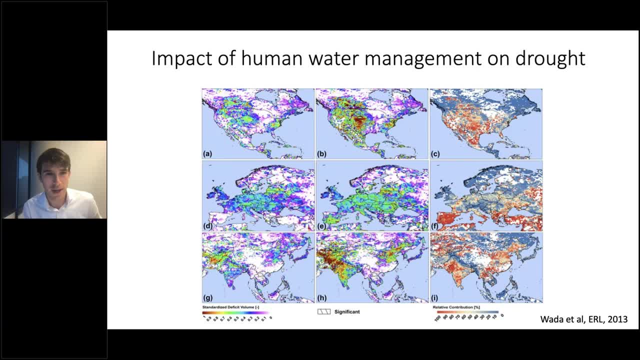 as a side project, which was a very fun side project to do, and what we did is we actually included humans in our simulations. so on the left- uh, you left three pictures for the us, europe and southeast asia. you see the natural conditions, the natural standardized deficit volumes, that's. 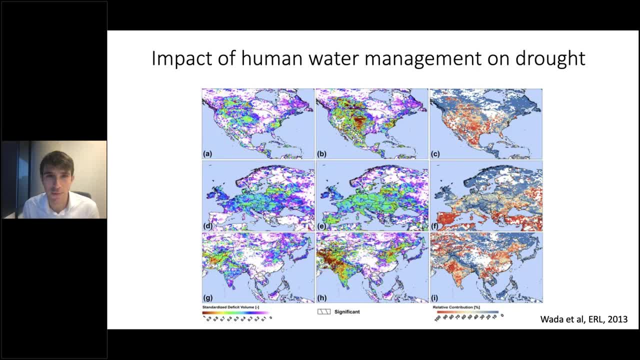 a measure of drought in the center row. you see what happens when you do include humans and their water consumption, their irrigation, their households, their industry, their livestock, and you see that the brown areas are popping, popping up, making droughts more severe for a couple of cases. and on the right you actually see a summary of that and you see the relative. 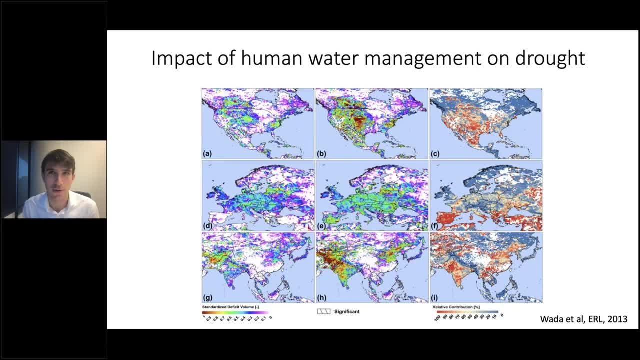 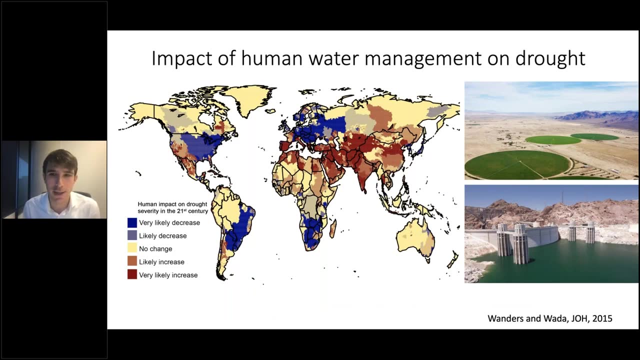 contribution of humans to the natural drought signal. so that's quite severe, and not taking that into account would actually, yeah, give you a skewed image of the future, because she and i continued in uh also still during our phds, uh by doing uh wonders and vadai in the journal of hydrology, where we actually 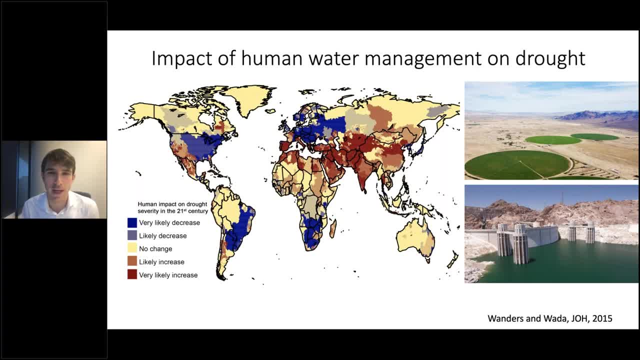 looked at the different components. we tried to include irrigation yes or no, reservoirs yes or no and how look how they will affect droughts in the 21st century. and all the blue areas show that human actions are very likely to decrease the drought impacts. and all the red 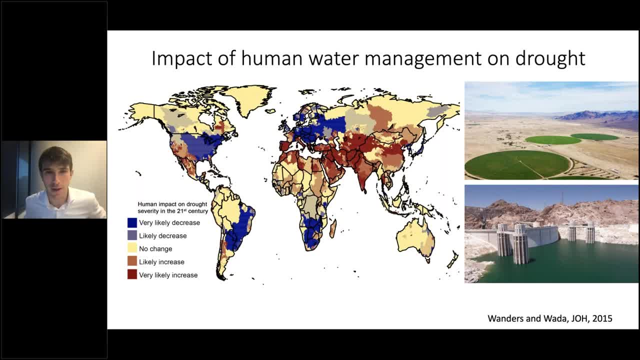 areas are very likely to increase the drought impacts. this is all an ensemble of gcms and models, but i just summarized in one picture here, and the blue areas are mostly generated by a smart reservoir management, while the red areas are often caused by increased groundwater pumping and irrigation and thereby leading to more droughts on the long term. so human water management does. 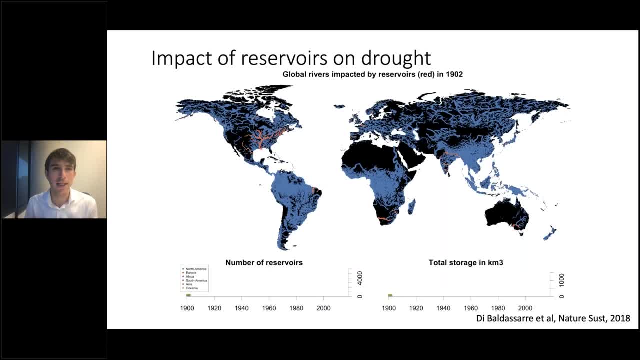 impact the drought here as well, and we can see that as well if we zoom out a bit. so here i made this animation from 1900 until 2010, from the top of our uh. we started together with giuliano de baltasare, who is actually giving the witherspoon lecture this year. we looked at the impacts of 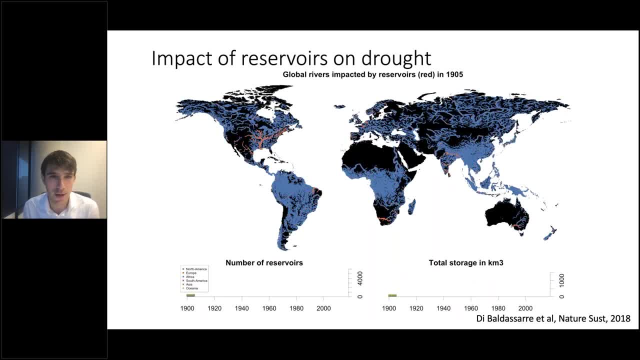 uh, on water use and and dependency of people. and you can see here in this animation just we. i only show you here not any results on on the paper, but i just show you how reservoirs impact major river systems around the world and we start out pretty much in blue and we end up pretty much everything. 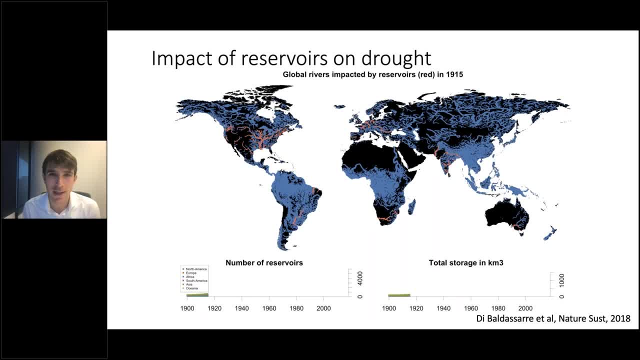 red, or at least north america and europe, and you can see that the percentage of global natural rivers is very limited at this point. and you see, on the bottom you see the number of reservoirs per continent and at bottom right you see the total storage in cubic kilometers. we had this. 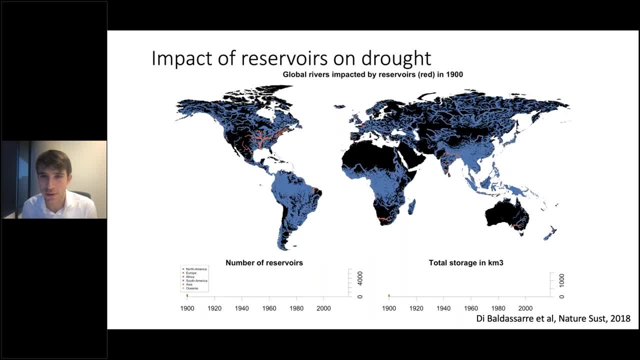 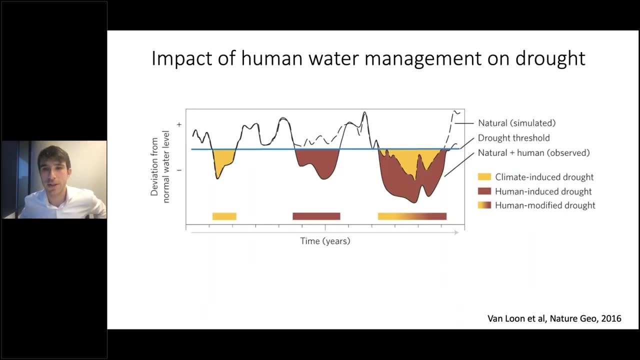 decade of engineering between 1960 and 1980, the two decades or where we can construct a lot of those reservoirs, but that has a major impact. i'm not including. that would actually limit your insight and knowledge of the system. anna van loon actually made a very nice graph on that. the nature: 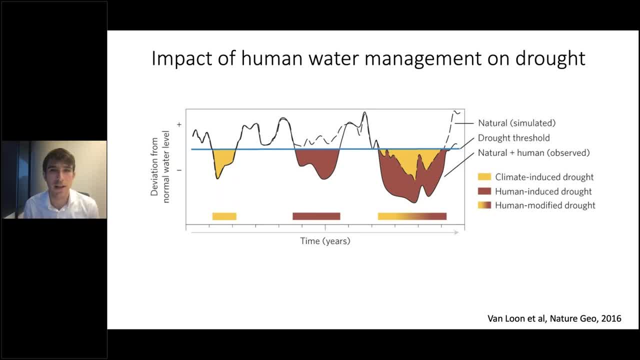 geoscience in 2016, where we say, like you have climate induced droughts, so basically only caused by climate, and you have, uh, human induced droughts that are just there because humans are using water or affecting the hydrological system in another way, and you can have, of course, have a human modified drought where you already have a natural drought. 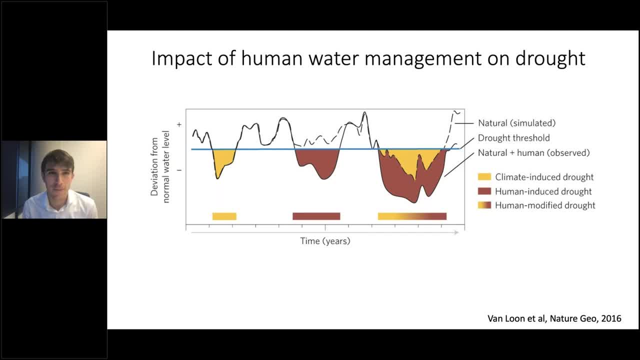 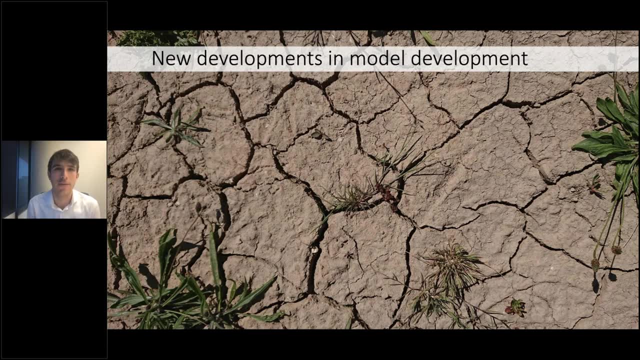 but you add more to that. so i wanted to actually not spend a whole historical, but i also wanted to go into the new developments and i put it here: model development, but new developments and i tried to highlight here things that i find interesting that are currently happening, uh, done mostly by early career. 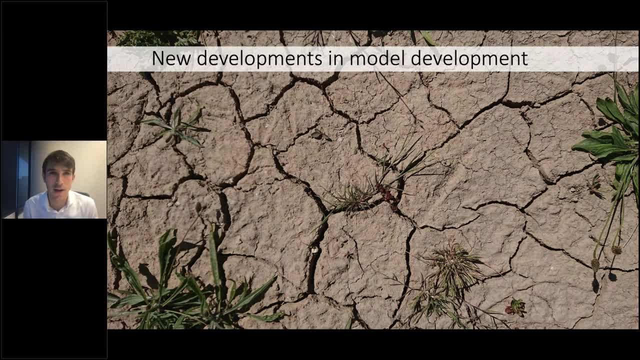 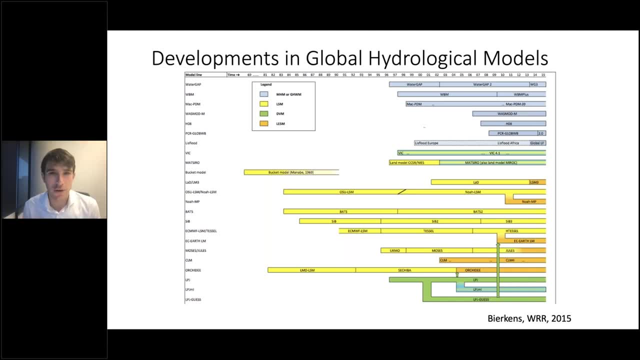 scientists, because i think there's some very exciting stuff happening in that regard and happening in that front. i start out with another non-early career scientist, but mark bieck has already made a nice graph- at least one i like- on how we've been developing global hydrological. 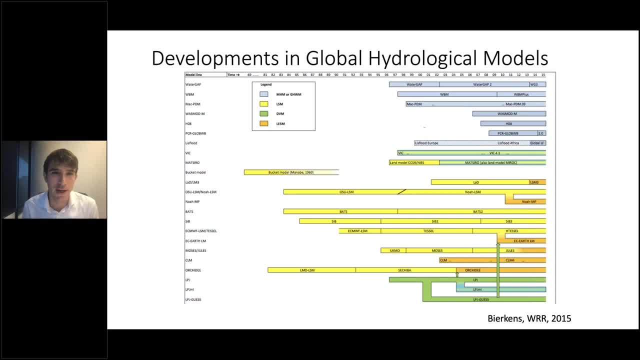 models. uh, through time we started with the very earth first bucket model in the 1969 by by the nam maname, and then actually we developed further and further and things become more and more complicated and on the other hand we have also included more and more models. so you see that. 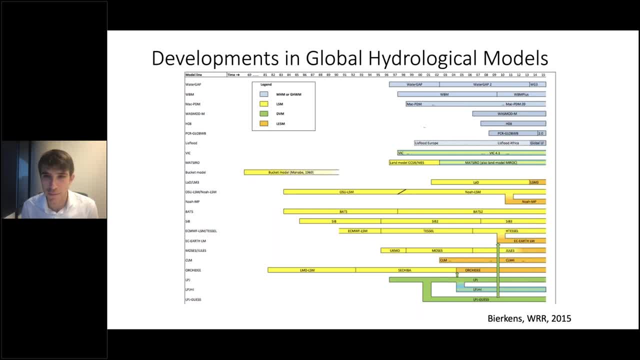 the number of models is increasing. there's some crossovers, some, uh, there's some change. some models become, uh, more hybrid and can deal with more things. uh, you have the typical on the top, the, the hydrological models, and then you have also more the land surface models and you have the. 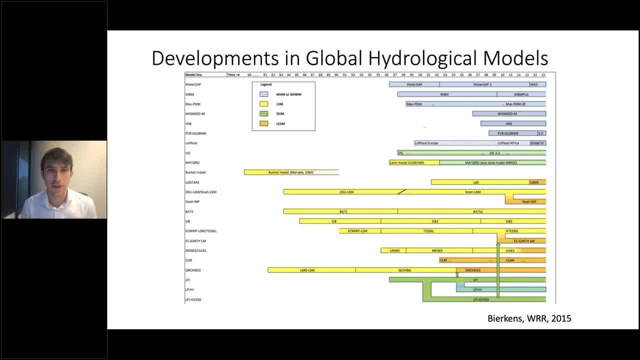 dynamic vegetation models at the bottom and you, you can see that uh, the, the, the, uh, the, the, the, uh, the. you can see that there's a lot has been going on and this crop only goes until 2015, but I'm I'm guessing until 2020. even more will be added and more new. 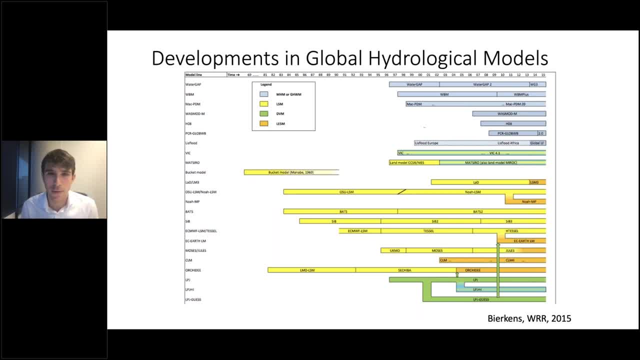 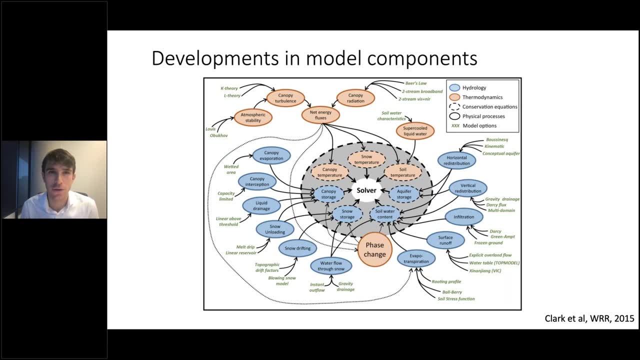 model, versions and components will be will be in there. one of the things I like is the approach by Martin Clark, where they actually try to have a soul or an environment where we can can exchange components and interchange different modules of models but- and thereby thereby looking and in standing- 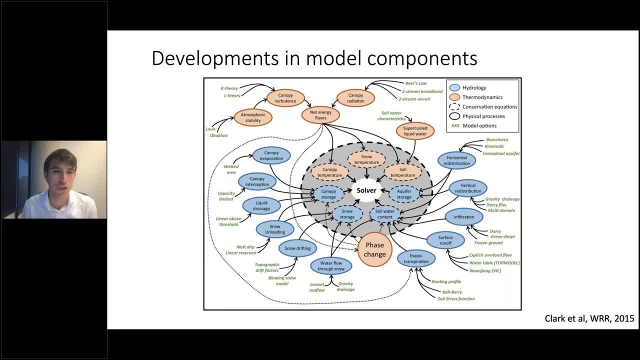 better the impact of selecting a certain model. it's been shown that the choice of model is not necessarily driven by the fact that you want to have the best model, but just by the fact that you can actually use it and run it and it started. and this kind of tools, as here the depicted, actually give you the ability. 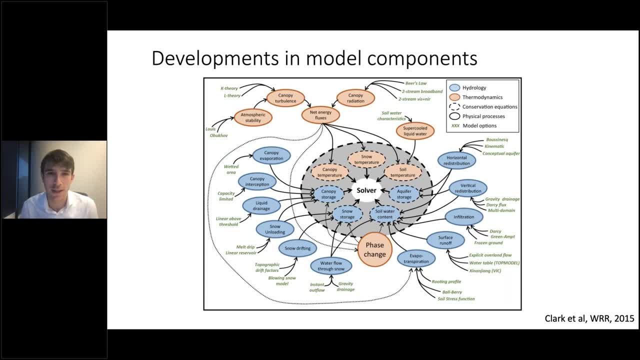 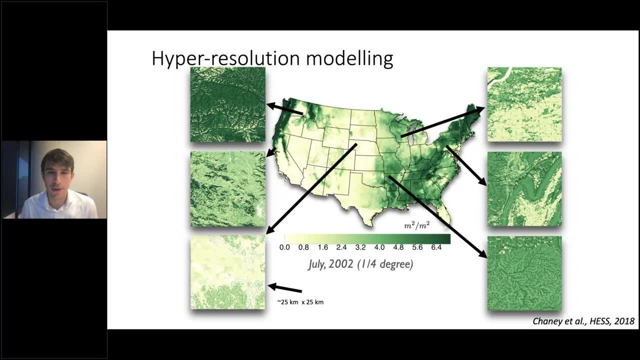 to actually change and adapt your model structure in a way that that actually is very suited for the things it should do. I want to start by into the new development section with hyper resolution modeling. I mean, it's the. the term has been out there for a while and it's been seen as a nice 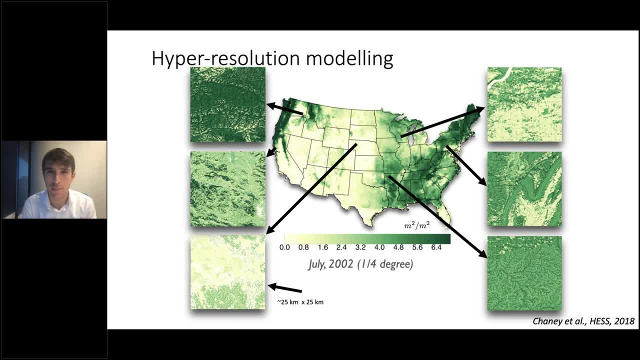 opportunity to provide more detail and a way pathway forward if we want to further understand the global hydrological cycle and the impacts of different components and- and what I think is a very interesting approach, the one taken by Nate Cheney, currently a Duke, who developed HRU kind of concept. 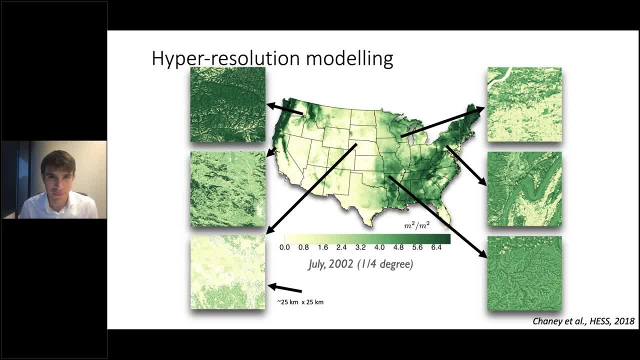 on top of a core scale, global, more global circulation model, and you can see here it takes one pixel and then finally make it way more, up to 30 meters resolution and simulation of, in this case, vegetation, and then you can think, of course, that's a nice, nice exercise, it gives nice pictures, you can see some. 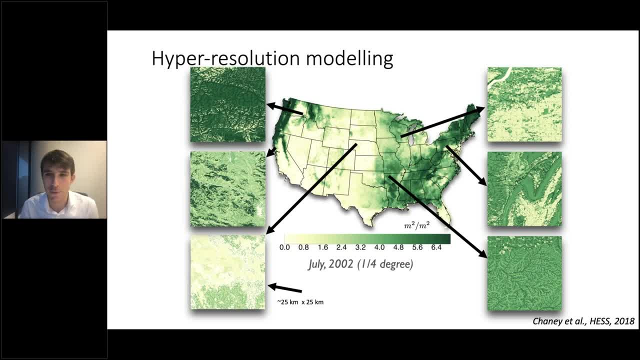 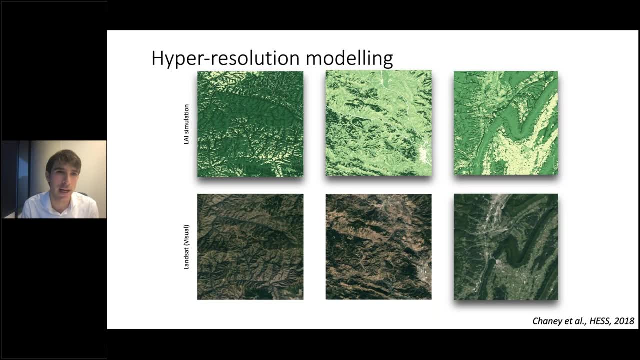 structure. you can clearly see some elevation impacts there. but actually what I find most compelling was- when Nate showed me this, this comparison between the LIA simulation, so leaf area index simulation, so the vegetation leaf density, and on the bottom, the Landsat area, so the top is. 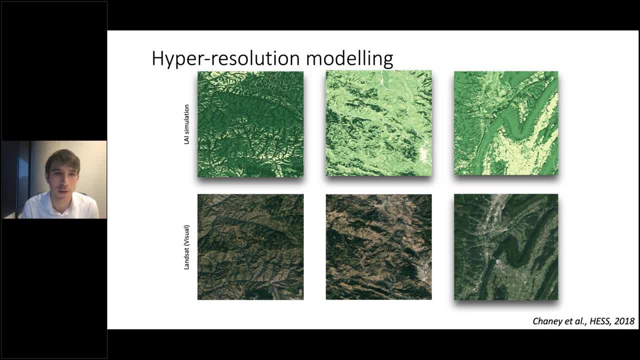 model driven, given by topography and other components, and then the model resolves how the vegetation should look and then the bottom row is actually what it is in reality, and I was quite impressed by the resemblance between the two two rows, and that actually gives me confidence that this is a nice approach. 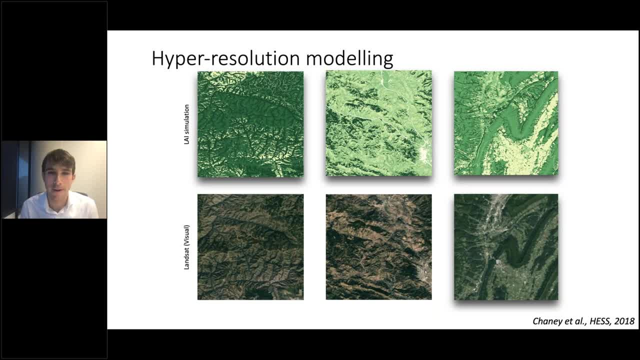 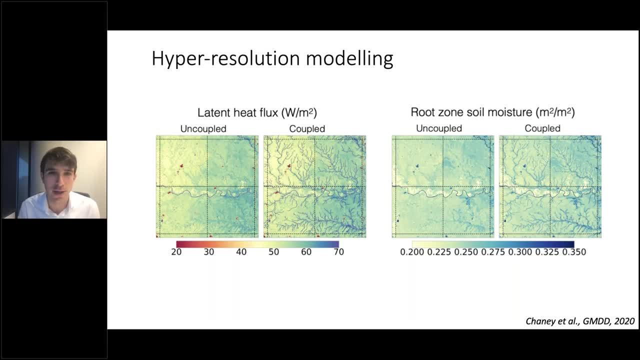 to to take and a route to take and apply. we recently published a new paper- I think it's still in discussion, so if you want to have a read, just go for it- but where he also coupled this approach to a more to the better stream routing network and what you see on the left, you see the latent 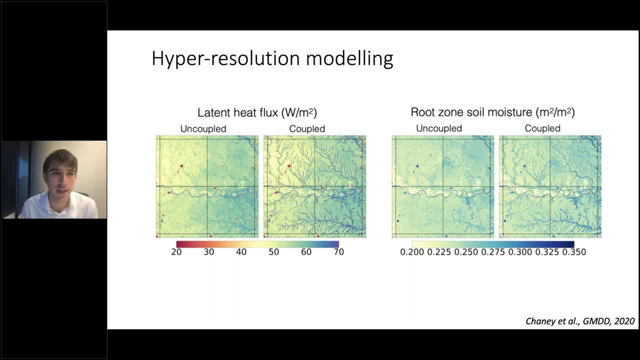 heat flux and you see his original 2018 work with. you see the stream. you see an uncoupled approach and then he coupled it with a more advanced routing model and you see more streams popping up. but you can definitely see the impact on the latent heat flux. 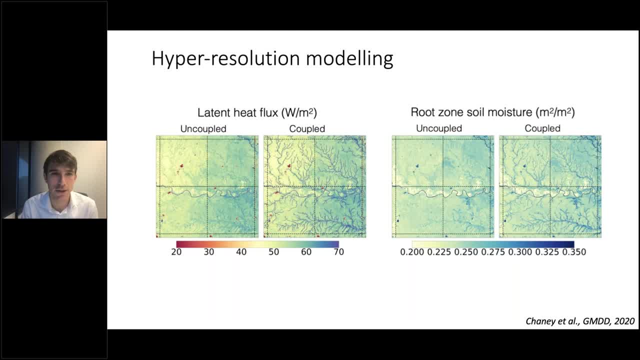 so there is definitely an impact of including this sub grid heterogeneity in your model simulations, not only in the hydrology, but also in the feedbacks to the atmosphere. on the right side you see the roots on soil moisture, and then here again you see the uncoupled simulation on the left and on the right to see the 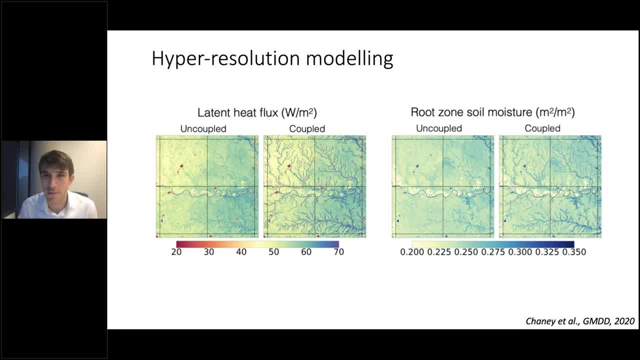 coupled simulation and you can clearly see there as well that by including that connection, you actually have an impact on on the roots, on soil, moisture and also the wetness close to the streams, and you could think: how is this related to drought? of course, but this is very important when you think of the 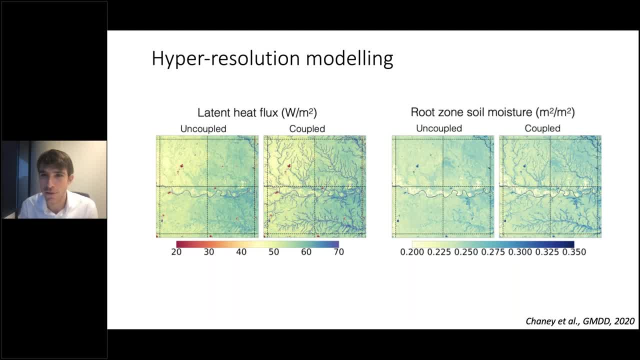 the long duration droughts and the the ability of nature to to deal with those, because if vegetation is close to those streams it is actually more resistant to those long duration droughts and and we might be able to survive these kind of aspects. so that's quite a very exciting uh development, i think. 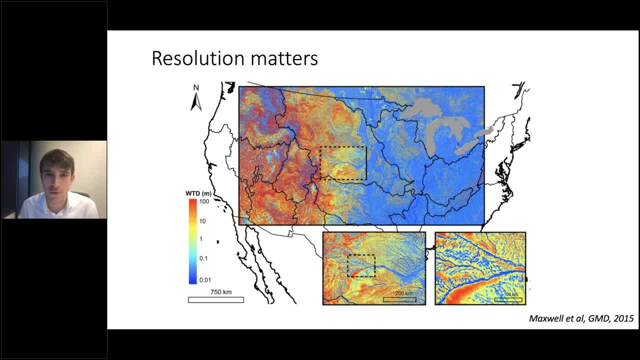 another exciting development that i uh i look to what a great enthusiasm is like the developments from parflow from reid maxwell's group. this is the gmd 2015 uh figure, but they uh parflow simulates and a very high resolution simulates, uh, the continental united states and i. 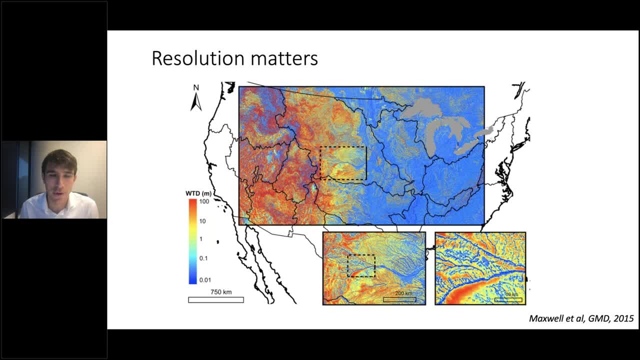 know that they can do more at this point, europe as well. um, by solving, uh, all these equations, not like in a traditional block type kind of way that global hydrological models do it, but uh, really solving the equations in this way, they can actually provide very nice. 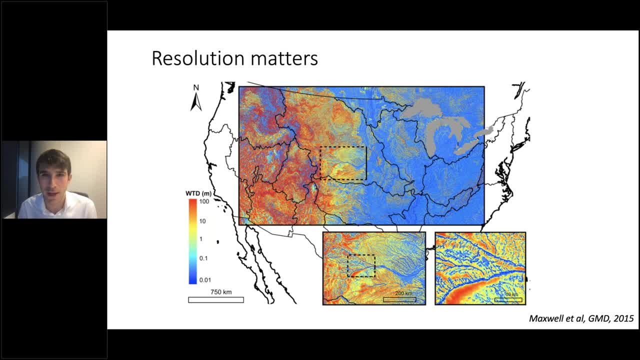 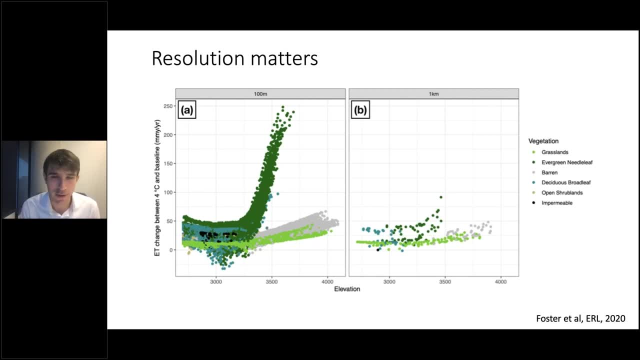 uh, simulations and not. i mean the simulations look nice, so that's a compelling selling picture, but also, if you look at, what does it mean? and this is work by foster at all in erl and this year, published this year, it also has an impact. i mean, it's not going from 1k. 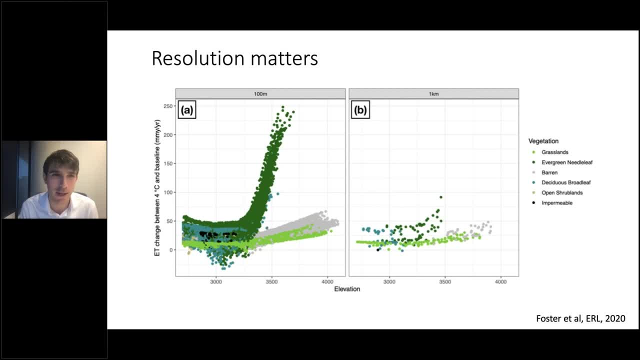 100 meters, that it's just nice pictures. it also has an impact, in this case, on evaporation, the change in evaporation between a four degrees warmer scenario and a baseline. i mean they simulated the climate change experiment. but if you do that on the left side in a 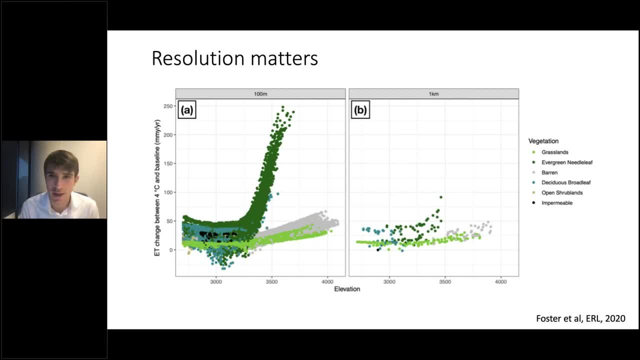 100 meter simulation. you can see that especially for the evergreen needle leaf, there's a significant impact on how that translates into the future. and on the right side you see a smaller picture. but you see you don't get those outliers that that are can be so important. 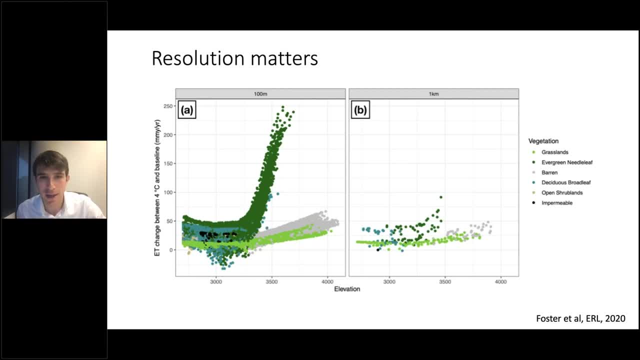 and especially when you're looking at the extremes. so i think uh that adding resolution is, of course, first of all, a challenge, but it also provides, uh might provide, new information that is much needed, especially when you look at these extreme uh drought events that are happening in the future. 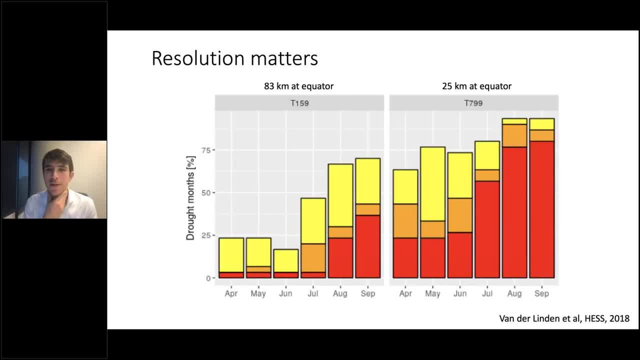 this is also actually confirmed by a different study by evelyn vanderlinde in hess in 2018, where she just looks at the impact of resolution on general circulation models. on the top left side you have the 83 kilometers at the equator courser model. that's a model typically used in the cmip5. 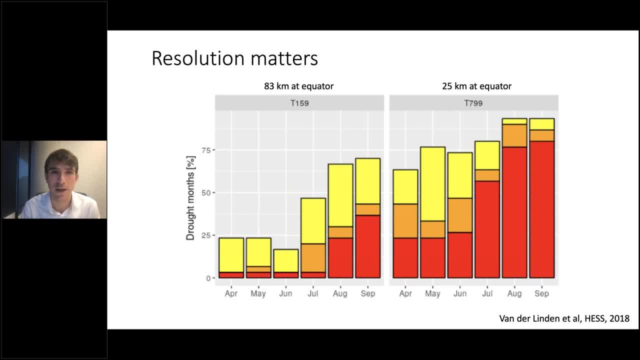 setup for the atmospheric people among us. t159. i've always had difficulties with this, so that's why i put the kilometers there as well, and on the right side you see a finer resolution model and that's even finer resolution at the current ongoing cmip6 simulations that we have. 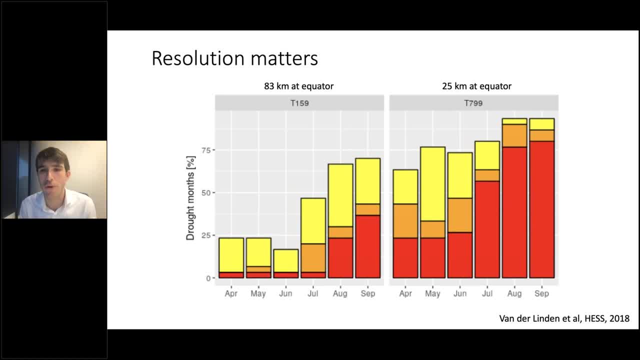 and you see the drought in months. so you basically see the more red, the more drought, and what she shows is that by increasing resolution, you actually get more drought with the same model, and whether or not that's true- i mean in this case it can't be validated, but that will definitely. 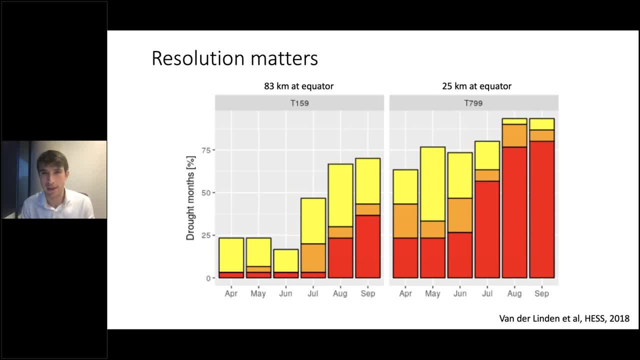 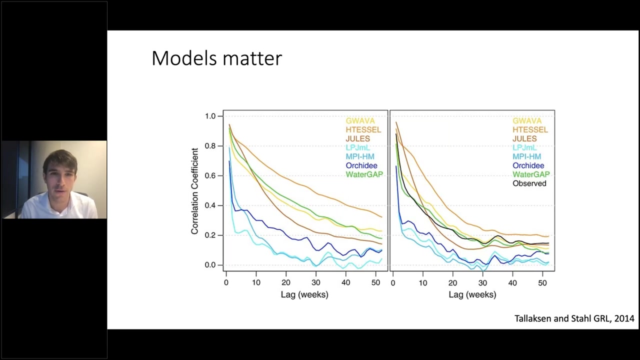 have impact when you look at climate projections and the ipcc reports. if we go to final resolutions, we might actually be able to detangle more droughts that are happening in the future than we, so our current estimates might be actually on the conservative side. then models matter as well. so, yeah, we often use a model, a hydrological model, but here i took 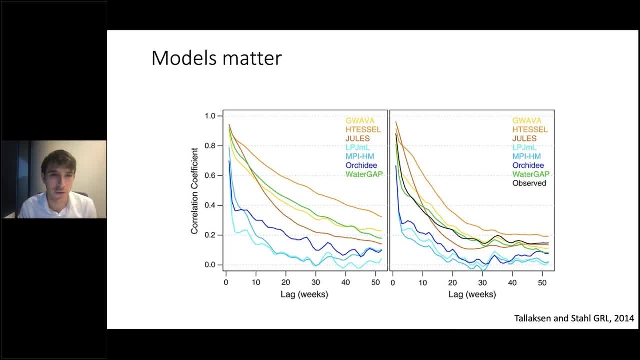 a graph from thalics and style from grl 2014. they looked at the autocorrelation of of certain models, and it doesn't really matter what which variable here, but what you see is that the autocorrelation drops off for some models very rapidly. so the memory in such a model? 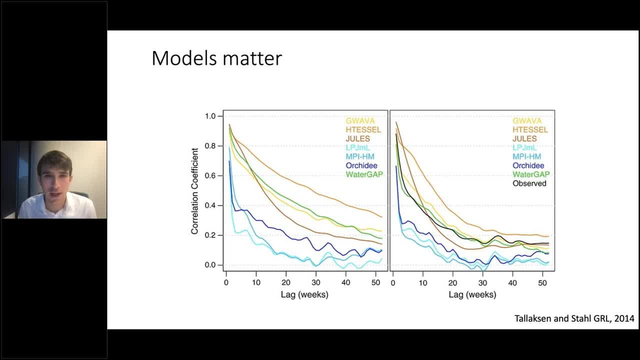 has a tendency to take only 10 weeks, something like that, while other models have a tendency to take way longer to to to lose that memory. and that's again important when you try to simulate processes, long duration, large extent processes like droughts that typically last for longer. 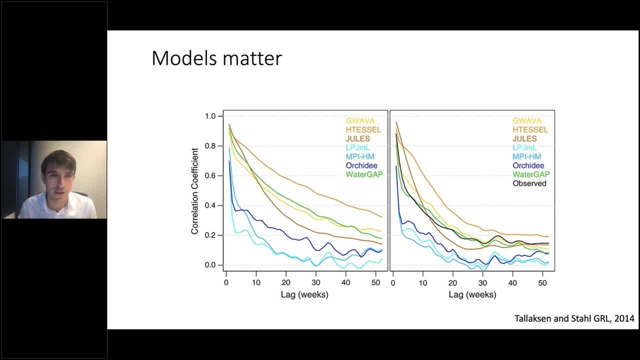 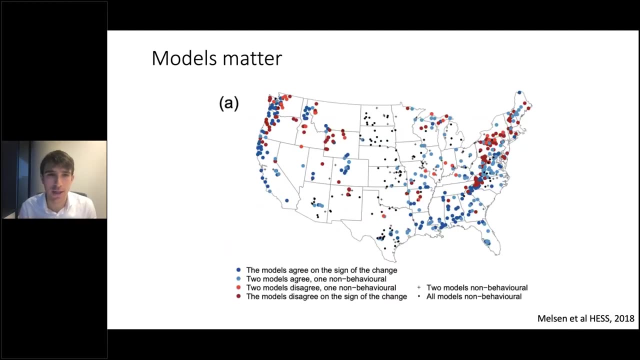 times, because if the model forgets about its earlier state faster, then the recovery is faster as well, while if the model has the tendency to slowly recover, that has a significant impact, and that's actually also shown by lika melza 2018, where she compared models, forcing them with. 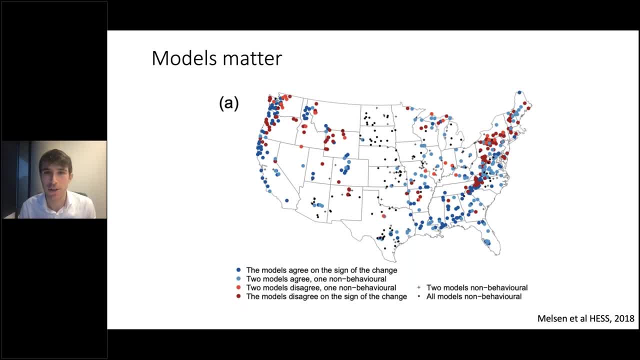 different, with different gcms, and see how much they agree or mostly disagree, and this is done for the us, and you can see that there's quite some disagreement between models, um, and, and therefore it really matters what kind of model you take, if you take an ensemble or if you take a selection. 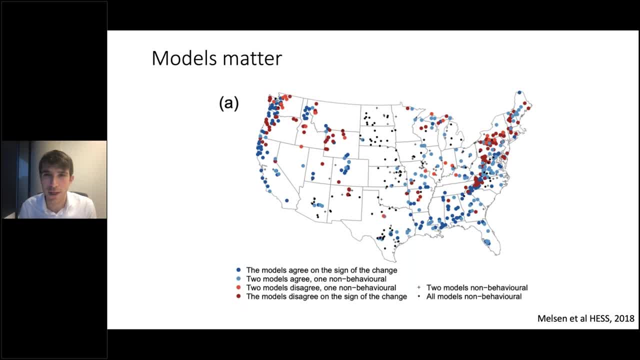 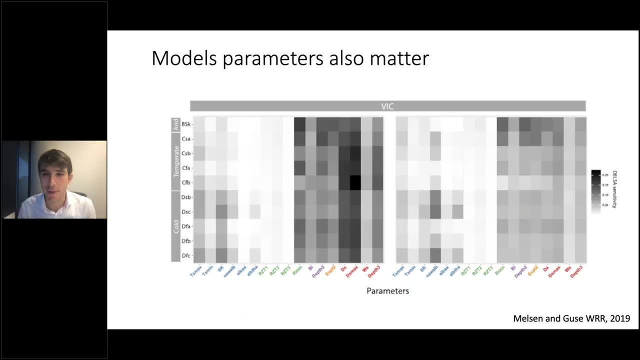 her paper actually goes into all the details of different gcm combinations, models, combinations and so on, but i thought this- this shows you just how important it can be to to be aware of these, these artifacts. then she also dived into in a later paper: uh, in the wr in 2019, also in the impact of 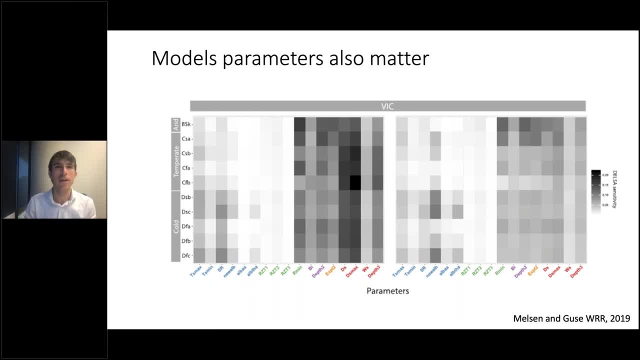 the parameterization and what you see, that not only the models do matter but also the parameters of the model do matter. so it's not just taking the, the one model. so i have fig here, uh, the variable model. and she actually looked at different climate zones going up into this graph and you see that. 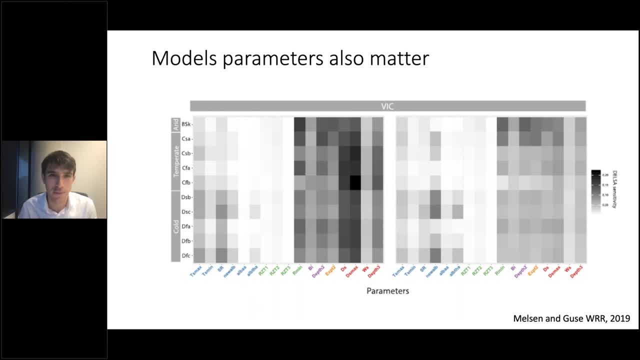 the sensitivity of the parameters for drought predictions she actually focuses on. drought is first of all relative, per climate, and second of all, you see quite that only some parameters do matter for drought, and i think that's an interesting finding when, if you calibrate models, what is your objective function and what do you try them to mimic or to reflect? 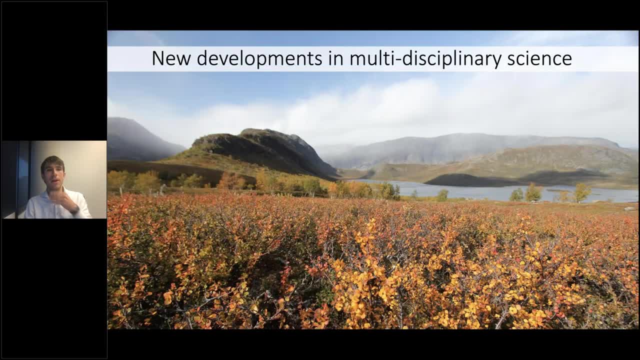 and then i think i want to move away a bit from the model development and look a little bit of new developments in multidisciplinary science, because i think a lot of the exciting developments are done in that field, where we combine our knowledge as an hydrology community. 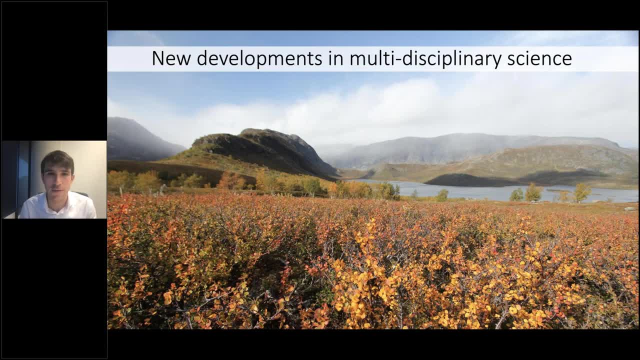 with the atmospheric community, the vegetation community or other branches at agu, and i think that that sometimes we can really push both our fields forward, and i've been really enjoying those com, uh, these kind of things. so i think that's a really good point, those collaborations as well, and i think that's also why i want to advocate for them here. so one: 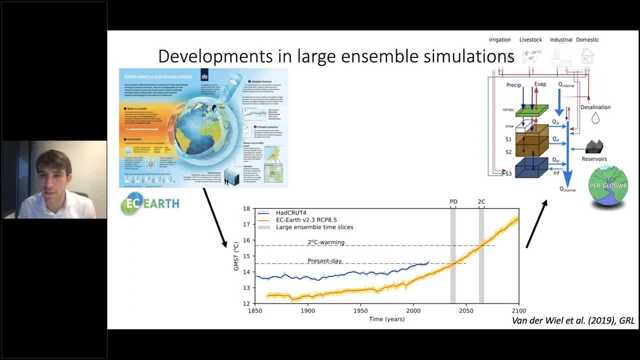 of them is uh, where we collaborated at kind of on the view from the knmi in a 2019 grl paper. in the atmospheric community, they have these large ensembles of where climate models are used to generate, in this case, 2000 years of weather events, and the advantage is that 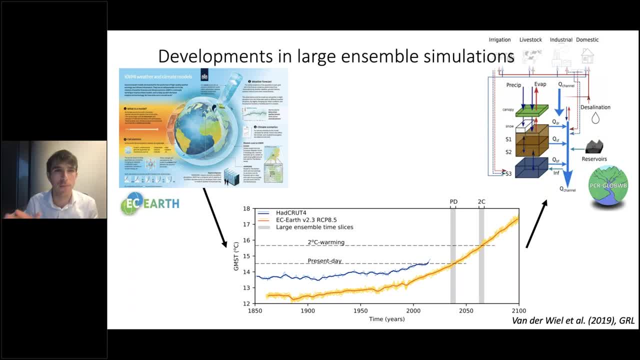 karen did this in this way, that such a way that actually the atmosphere was coupled to their land, to their ocean. so it's a really a system that is capable of reproducing extremes, physically extreme things, and by using a dynamical model we don't have to rely on. 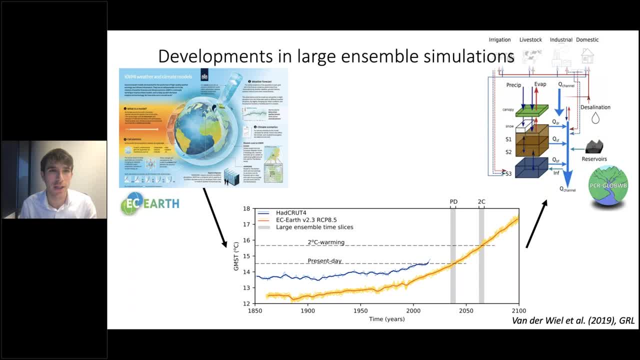 the statistics. so the model can theoretically go everywhere, as long as the the patterns are there. we looked at the present day in a two degree warming climate, so that's on the bottom left, just to compare the differences. and then we run it through our global hydrological model, pcr, glob. 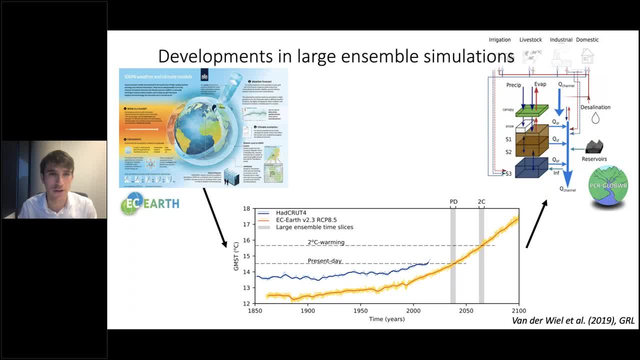 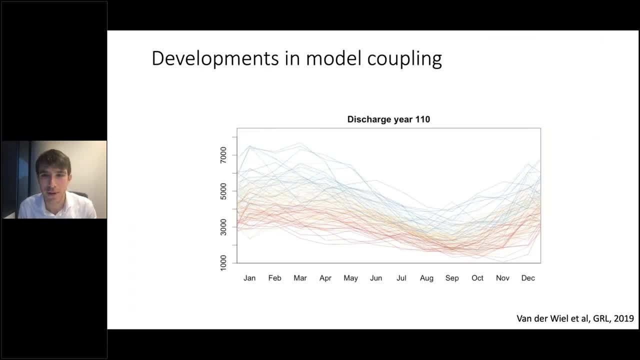 to generate global discharges around the world and look at, look at the extremes and without going into all the figures in the paper, I think you you can pick those up yourself and read it. I want to show you the impact of using 2,000 years. 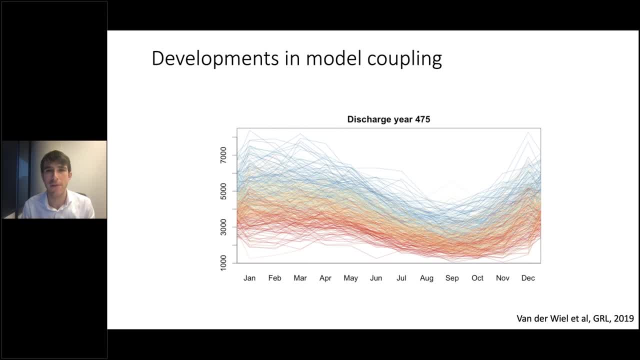 and not a hundred years, so the simulation starts by adding five years at a time, and this is for the River Rhine, which is a Dutch River. but yeah, since I live there, that gives me some reference. and I color-coded all the red lines be to be the very the driest of all and the blue lines to be the most. 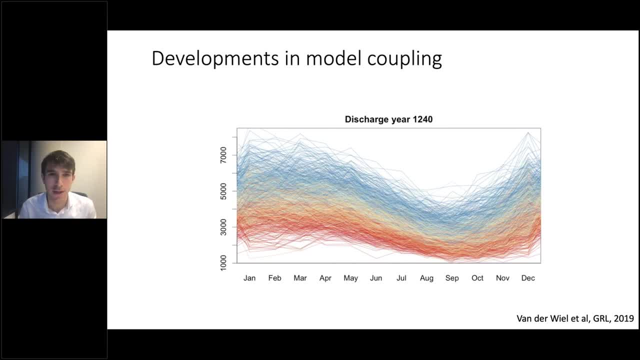 wet of them all. and then the yellow is a little bit in between. first of all, you see that some of the red lines start out low and go high and go low and they go over over the place. some of the blue lines are the same, so it's not like they. 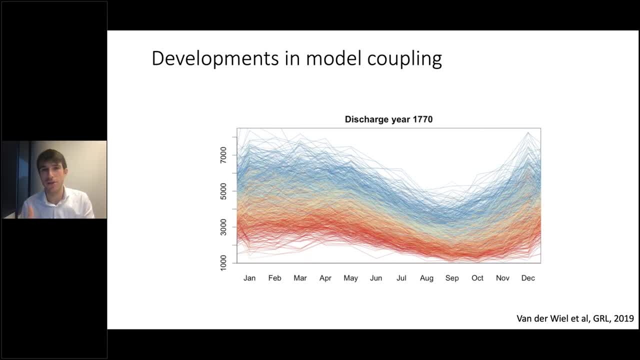 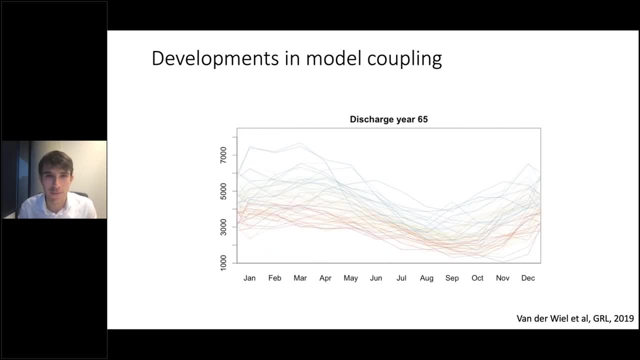 always stick in their own zone, so you can't say, oh, this year starts out dry and it's gonna be a dry year after all. and second of all, if we start the animation again, what fascinates me is that, even after like a thousand years, that we already had adding new ensemble. 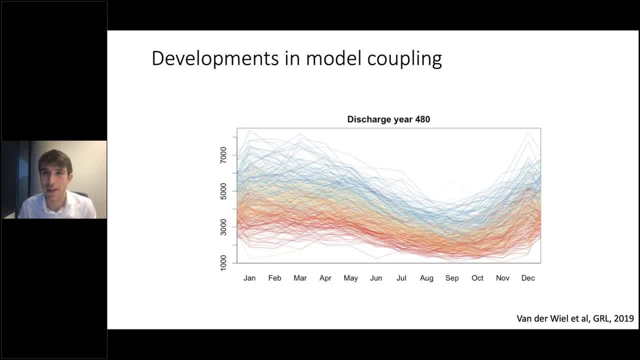 members will still give us events that we have not observed before or simulated before in this case, and also, if you go and look into the distributions of those events, they don't tend to follow that and always tend to follow the generalized extreme value distributions. so actually looking at, 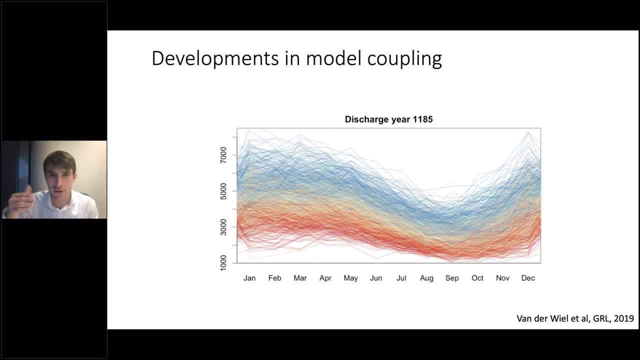 those extreme tales can give us a lot of information. so now you can actually see. if you look at the high end specifically, then you can actually see that some of the lines pop up now like extreme events that not have not been observed before. and of course, this we, this is not the. this experiment is not. 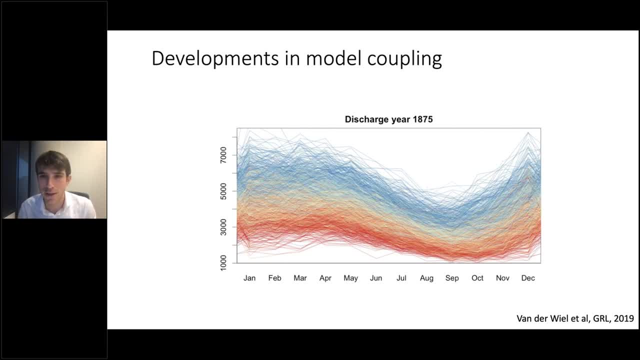 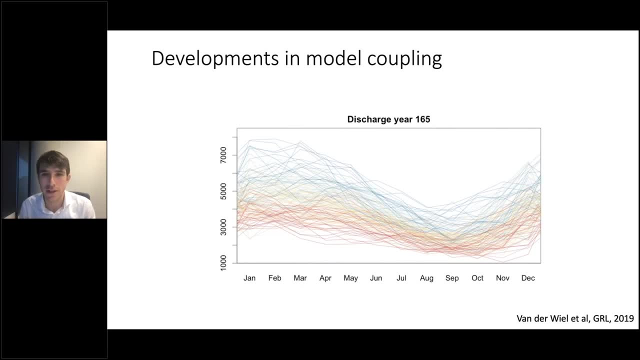 there with the aim to look at the one in two thousand year event, because the chance of that happening are very slim. but it does give us the ability to generate twenty one in hundred year events and look how they, what kind of patterns they might have in common and what kind of predictor they might have. 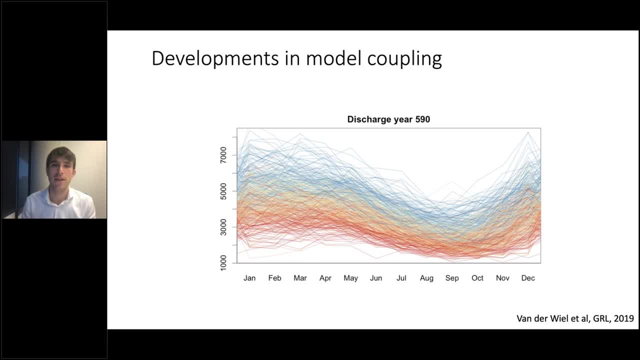 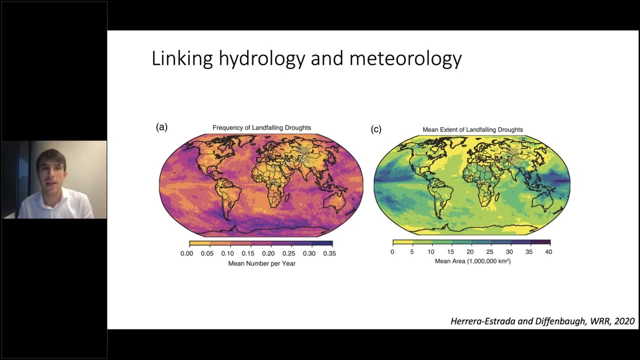 and how we can prepare better for those, and i think this is very exciting to exciting new thing to do by combining atmospheric science with with our hydrology knowledge and and looking and understanding together. another interesting thing is linking hydrology again to meteorology, and this is a paper. 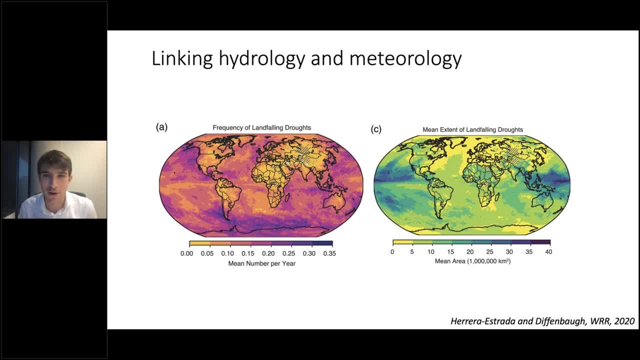 by Julio Estrada and Noah Diefenbach in WR this year, actually recently published, I think a couple of months ago, and they look at landfalling droughts and when I first read it I was like landfalling droughts, but it's basically. 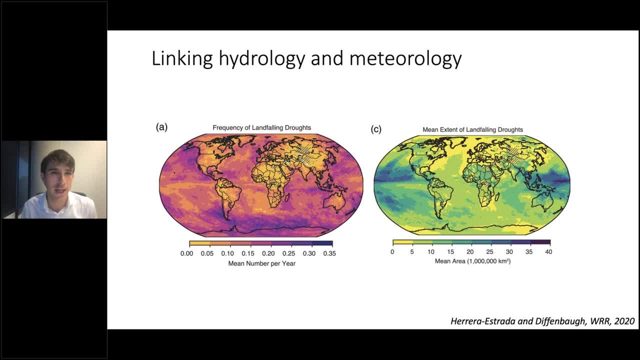 droughts that can be predicted by oceanic anomalies between precipitation minus evaporation and they actually find that most of the severe droughts or a lot of the severe routes are actually coming from the ocean and the exact mechanism. they don't go into detail on that, like what could be the predictive. 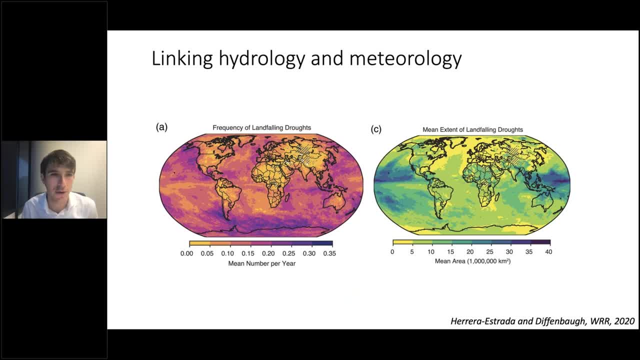 courses and and so on, and we've long known that ENSO and El Nino have an impact on on drought frequency. but this connection with the ocean is quite interesting and they track droughts through the and over land. and I think that this is just by looking at these other sources. 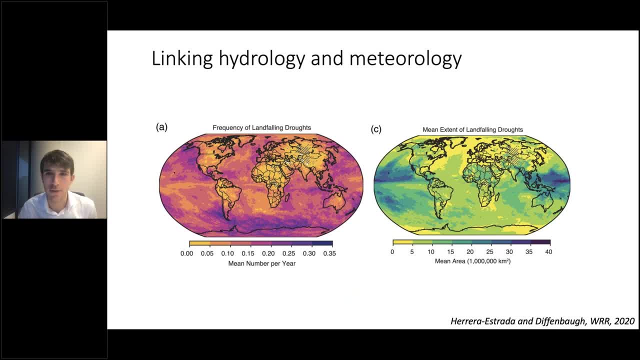 of predictability is quite an interesting way. you can also see that of on the right side. also on the left side you see the frequency of the landfall in drought. so how many you have per year and you can, as you can, expect on the west coast. as you have more of those, then you have in the interior of some of 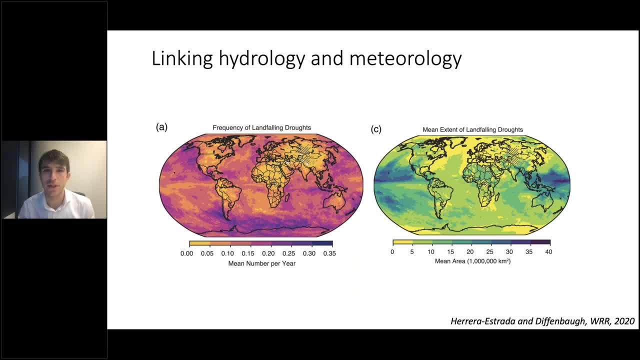 the countries and also the extent, so the size of those droughts, and they actually tend to be quite, quite big. Julio already showed in an earlier paper that you can actually predict droughts by tracking them over land. so, and I think this is a nice add-on, something that that needs further study, but it's. 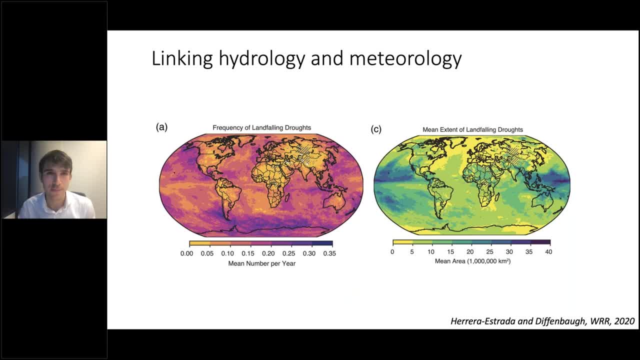 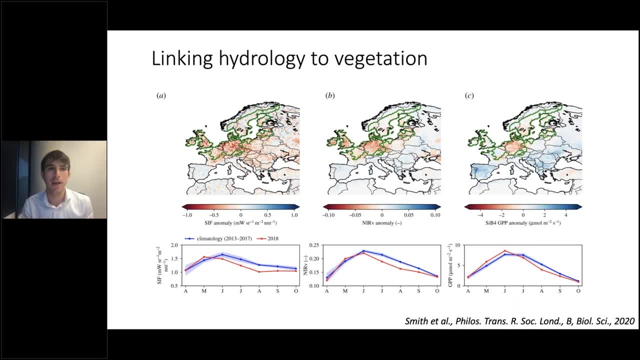 very interesting. first first approach here- I guess then some other things- is linking hydrology to vegetation. recently we've been coupling our hydrological model to a dynamic vegetation model and showing what the impact is of the drought with and without these coupling processes for the, the dynamic vegetation model, and you can. 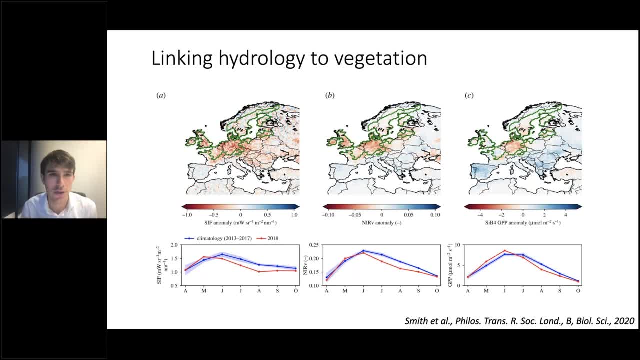 actually see. that not only does it improve the simulations but it also shows impacts on the near infrared and and the Jeep, the carbon production or the carbon for gestation in simulation. so for linking our hydrology to vegetation dynamic models, that might have a different simulation of the 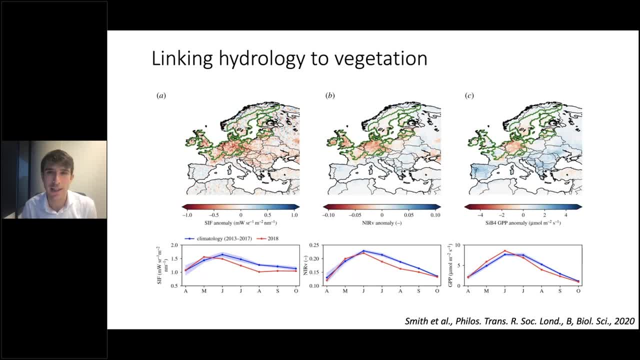 unsaturated zone and certainly the groundwater actually causes a different result in terms of carbon uptake and other fluxes to towards the atmosphere and linking our fields there. I think it's very exciting, especially also if you look at the drought recovery phase, where a lot of the hydrological models will just have vegetation that magically evaporates. 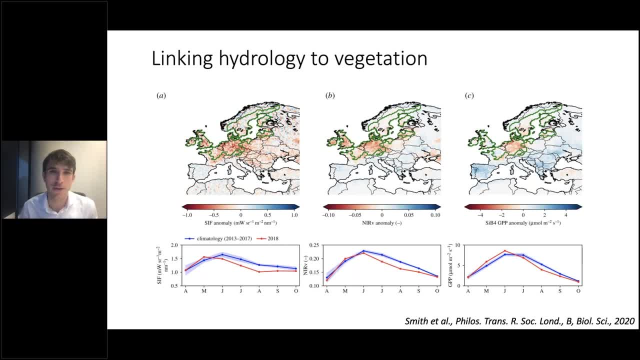 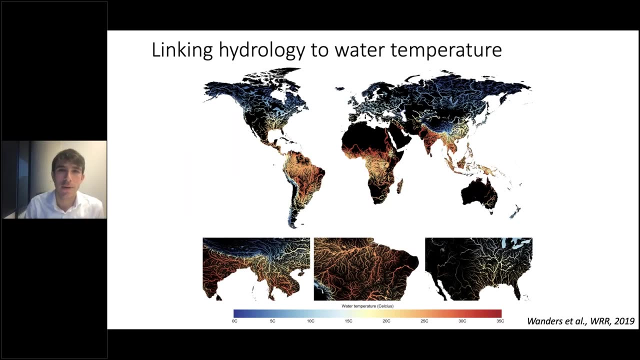 water again as soon as it has has water, because our vegetation is often not dynamic. and well, in this case is by coupling the two. we can actually incorporate processes like leaf shedding and so on. then another thing we've been developing, utrecht, is linking hydrology to water temperature and of 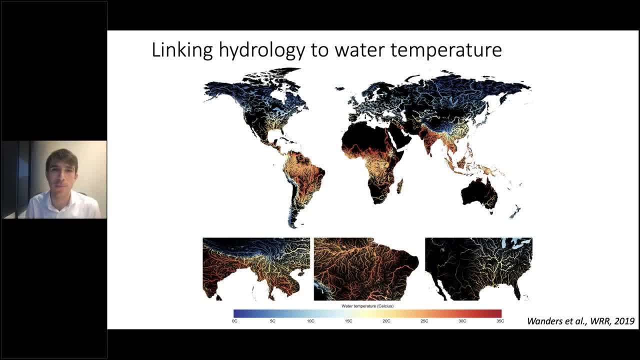 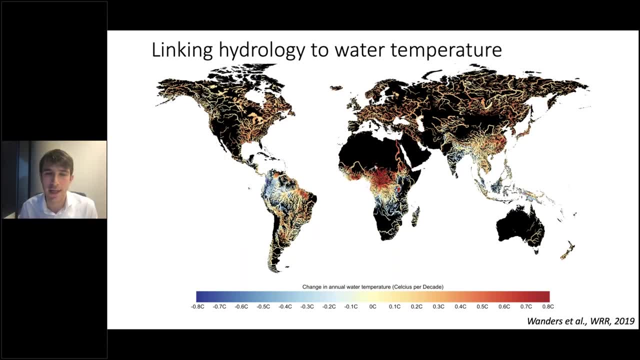 course, water temperature is a component of hydrology, but it's more and more used by other disciplines. so here I have the: the annual water temperature change in the decades over the historic period. but we we published this paper as we wanted to see if we can do this. but most 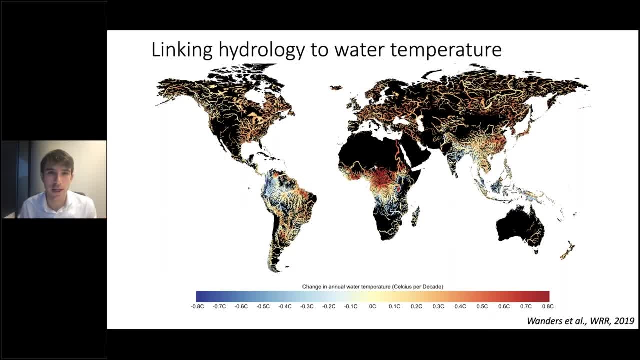 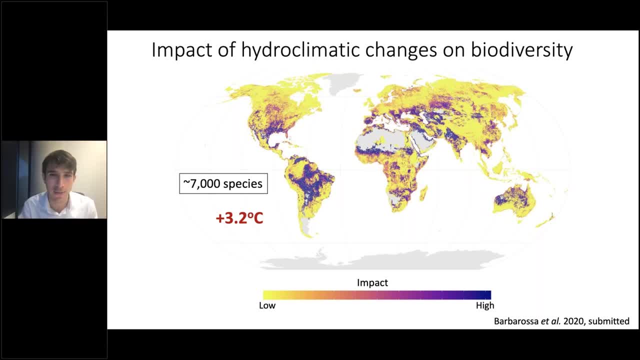 of the interest actually comes in the water and in the system, and so we want to be able to show you from different communities, like people that study biodiversity around the world. so we teamed up with valerio barbarossa in nijmegen, also in the netherlands. this is a work in progress, but 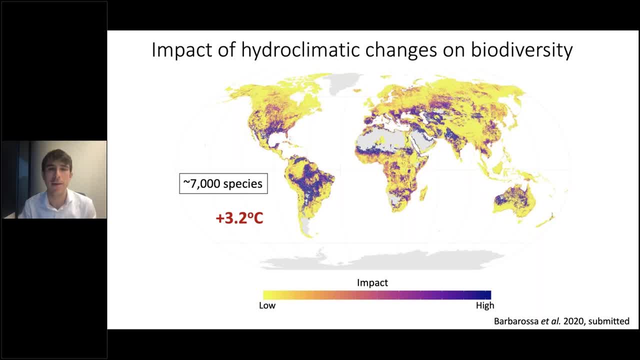 it's actually submitted, actually- but the impact of. they look at the impact of water temperature change and discharge changes on fish species and they used around 7 000 fish species around the world. so you see the world here again and where everything is yellow, the impact of climate change. 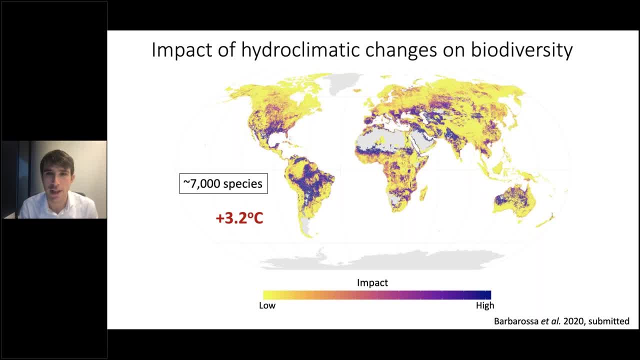 of, in this case 3.2 degrees warming is not that bad or it's low. i would wouldn't say that not that bad, but maybe low, and where the impact is blue, it's very high. and they actually have lab experiments where they professionally kill fish by raising temperatures for the fish species and seeing when. 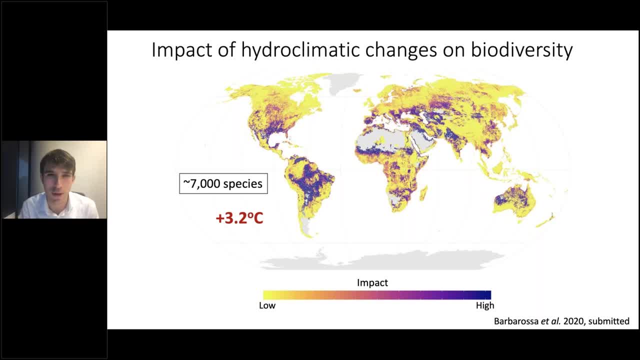 they die and they give. that gives them their comfortable niche. we know where those fish swim in which rivers, so we actually can see if this river system warms up more than a certain amount of degrees of temperature. so we can see how much water we have and we can see how much water we. 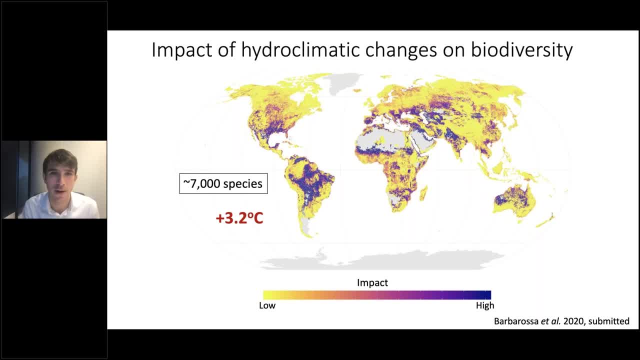 get, but at least celsius. this fish won't have no existence here anymore, and that's very exciting work, and we've also been teaming up with other uh groups around the world to, to, to look at this kind of thing, then invertebrates, but also fish species in this case, so very exciting, if you look. 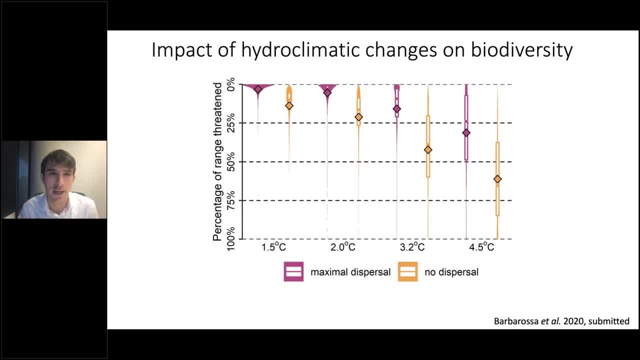 at the um, the summary of that work by valerio, you can actually see that if fish get the opportunity to have dispersal and so they can swim to a different river, then they are actually a little bit better off. but still, if you look at the 3.2 degree warming- 20 degrees around the world and we see this fish now swimming. Okay, is that clear? that completely same thing, it just coming to different places on that kind of. If you look at the fish, five years ago this fish actually would have to have 4 degrees. So by covering the fish, the gills are different in with water temperature. 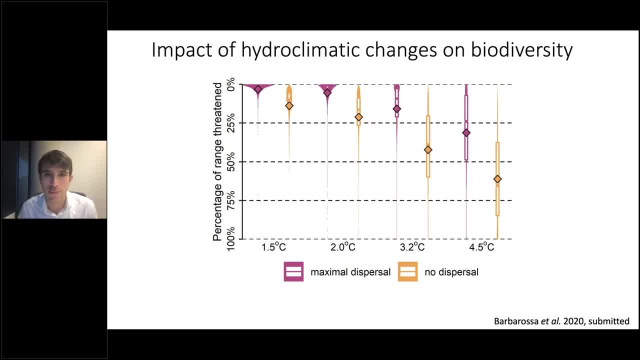 warming scenario, you go from 40% species loss to something like 20% species loss and 20% species loss around the world for all fish species is probably not a good thing, but it is very exciting to collaborate on these kind of things, although the reports or the yeah, the findings might not always be very happy. 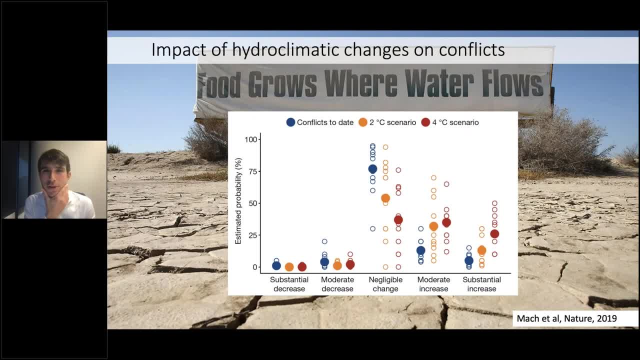 and positive, and that especially is true for the next topic they've been studying in here in Utrecht together with Sophie de Bruijn and Janus Hoog, two postdocs. we actually look at the impact of hydroclimatic change and conflicts, and 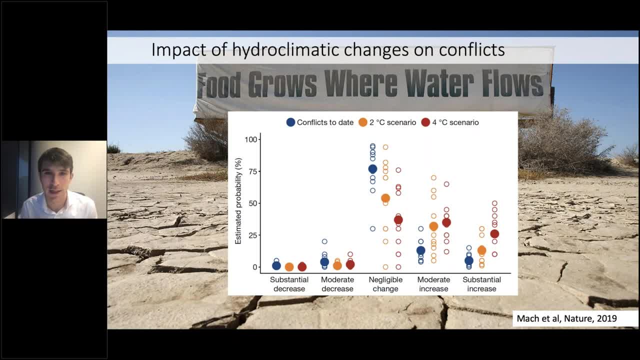 this is a paper by Machetel and Nature in 2019 and actually they interviewed a lot of experts in this topic and they said: what do you think happens with conflicts to date and how are they related to climate? most of them agreed that currently climate is not that big an impact on conflicts, but they expect. 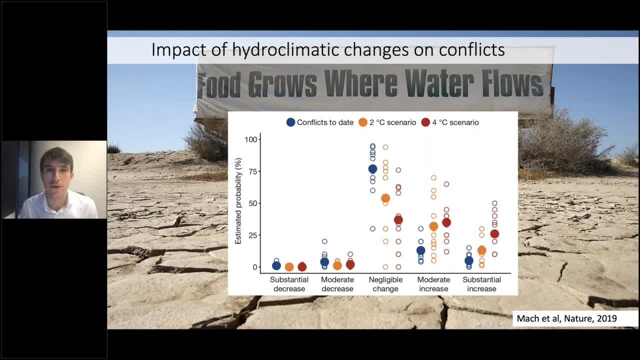 a moderate increase to substantial increase when we go to two degrees or four degrees global warming. so that indicates that and I think you can also see that in a lot of research programs around the world- that climate change is expected affected will affect conflicts in the future, is at least expected to do. 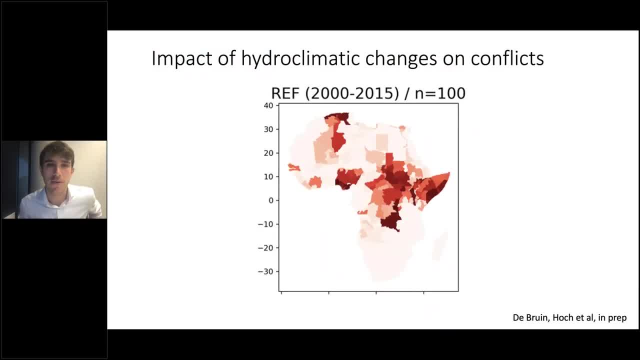 so this is our. so we try to simulate this now for Africa and try to get get a model to actually link climate to conflicts and also other socio-ecologic factors. this is still work in progress. you can see that there are a lot of studies that have been done on climate change and other socio-ecologic factors. this is still work in progress. 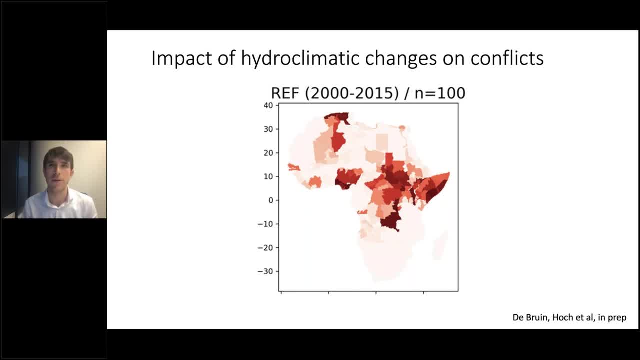 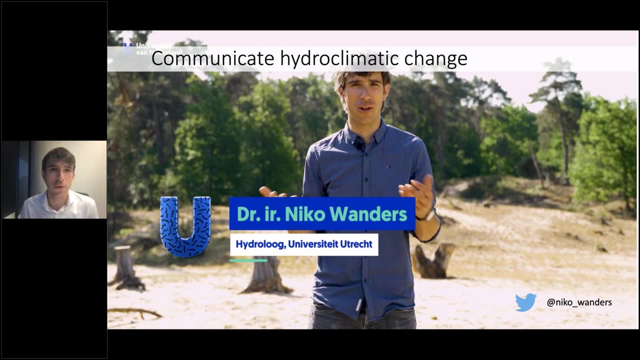 but exciting to to look at these other avenues. then I want to go and end this by going to a little bit more personal message. I mean, this was all very science and I think there's a lot of exciting things, but I think as a scientist we also have the ability, the duty to communicate our science and especially 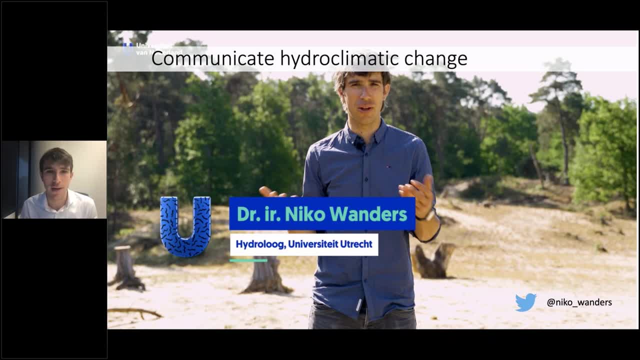 when you talk about hydroclimatic change- droughts, floods, climate change- do it on Twitter or in media or even give school lectures to kids or something like that. I really enjoy that last category. kids have are very open and their questions and they're also very honest in their opinions and I think it is our duty, even though it's. 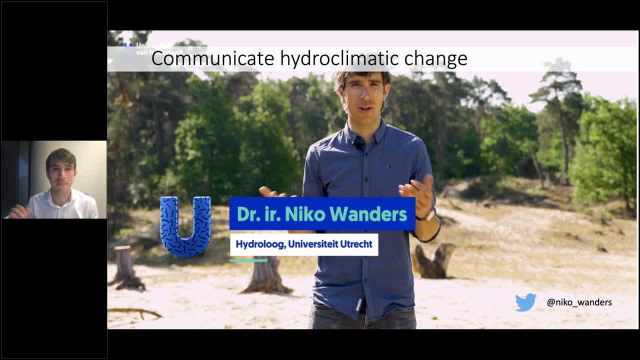 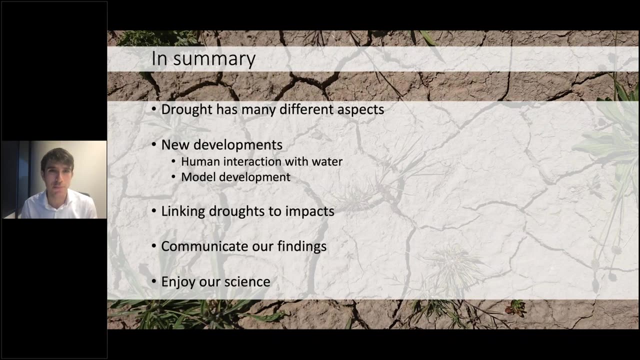 sometimes difficult and you might have haters around the world- to communicate that, your findings, in a nice way and try to say what you have and how we can prevent some of the impacts. so in in summary, drought has many different aspects, many different phases. there are different. 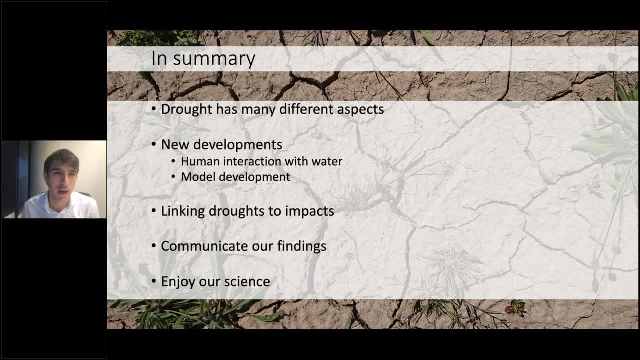 ideas and I think there's a lot of exciting new developments happening in human interaction with water. the model development so we better understand how our models affect the drought impacts. the link from droughts to impacts actually so linking the physical phenomena to underground impacts that bother people. 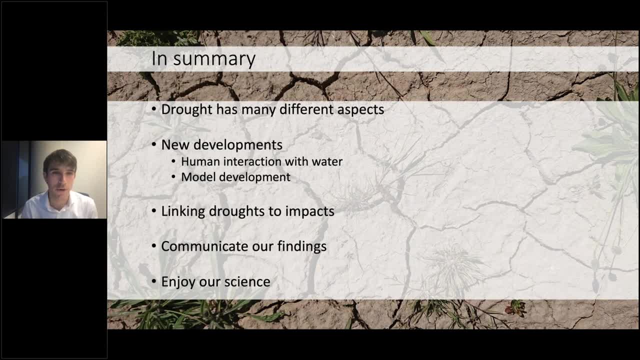 like crop loss or conflicts, and we have to communicate our findings. and I want to end on a very personal note- and I think we should also enjoy our science. I think that's something I did. I think I have an awesome job here on the left side giving. 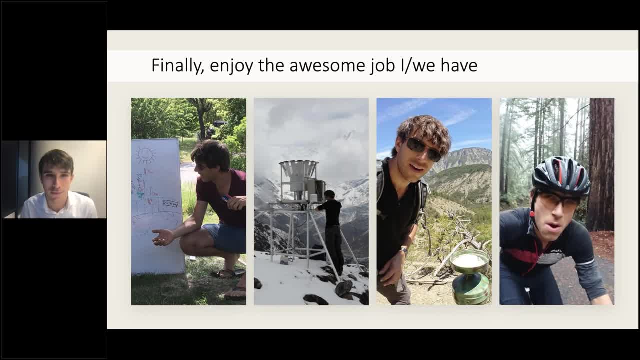 lectures in the fields: repairing a meteorological station in Nepal at 4 000 meters reading a precipitation bucket. then at the right side, you wouldn't say so, but that's AGU4 meeting last year. um, and I think- and I do that with other scientists who couldn't- can't be on the picture because of 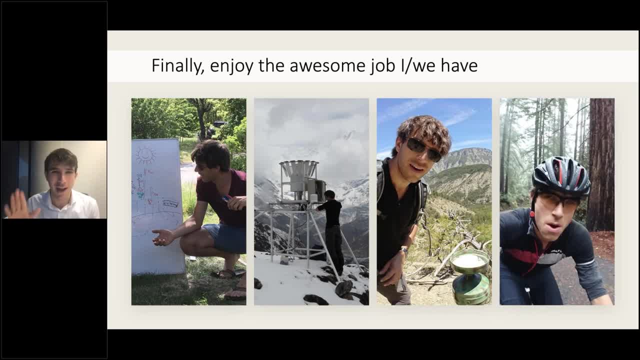 European law, I'm not allowed to put them on there without their consent. but I I have amazing friends around the world um join me in some of these adventures and i think i'm very grateful, uh, that i can have this job and do it and give this lecture now to you. so with that, i would like to thank you all. 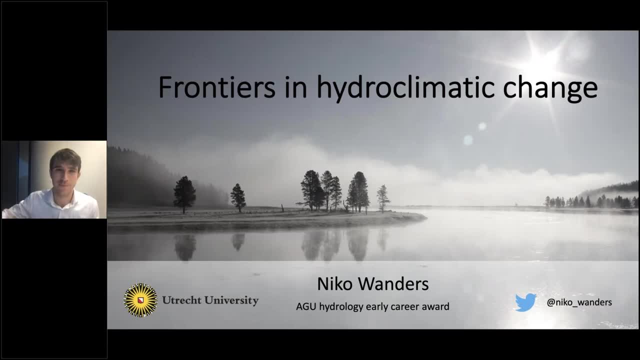 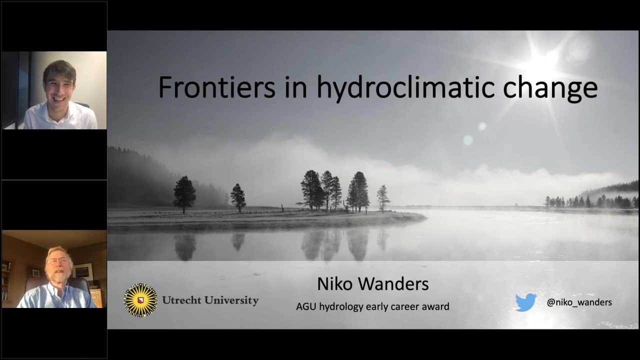 and i'm happy to take any questions. thank you, nico. thank you for communicating your science in a wonderful way and and still having fun with what you do. that is great. it's been part of my life as well. we're we're open for questions, so please, thank you. let's give a round of applause. 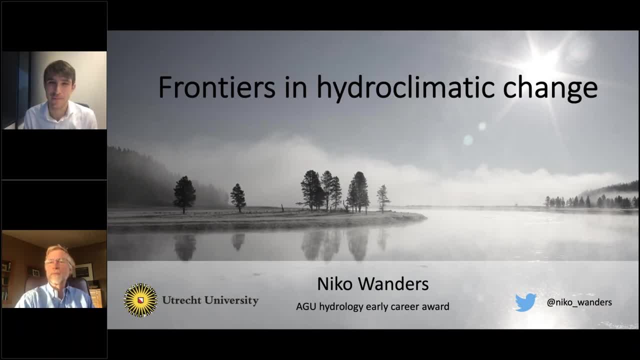 virtually to to nico. thank you and um, please type your questions into the question box. we have a great, uh, have a large number of you out there, so looking forward to hearing from you. um, nico, i have. i have one question, maybe to kick things off, which i found interesting. so i found all the talk very. 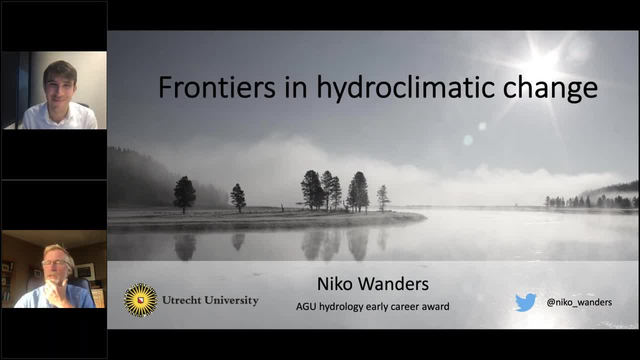 interesting. but when you were talking about linking hydrology to other disciplines and coupling with vegetation modeling, so so bringing the vegetation modeling community in the, the ecology community, if you will, with the hydrology community, and- and i you said so- you know we treat uh leaf area index differently than a, than a vegetation modeler would there may have a. 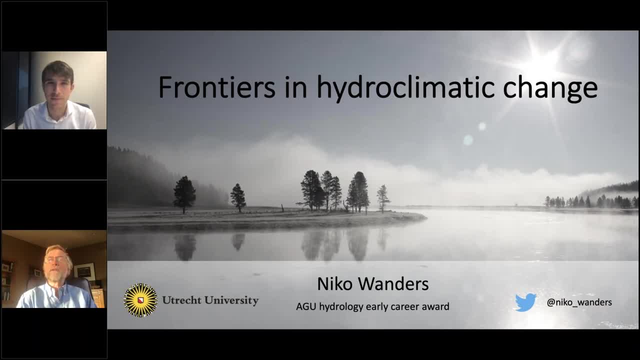 a different algorithm if you're going to couple those two together, as you did, how do you decide who wins, if you will which? which community wins in, say, how i treat soil moisture or how i treat leaf area? and because are you making a qualitative judgment that if it's green, then the vegetation? 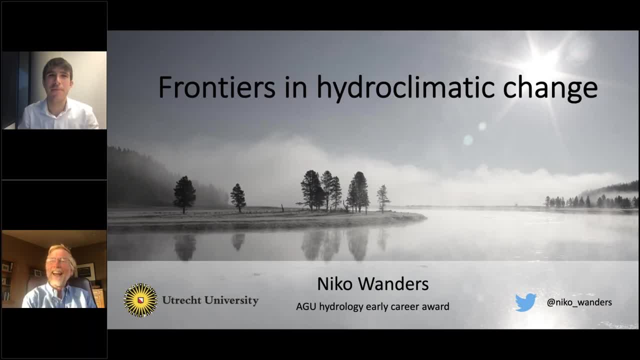 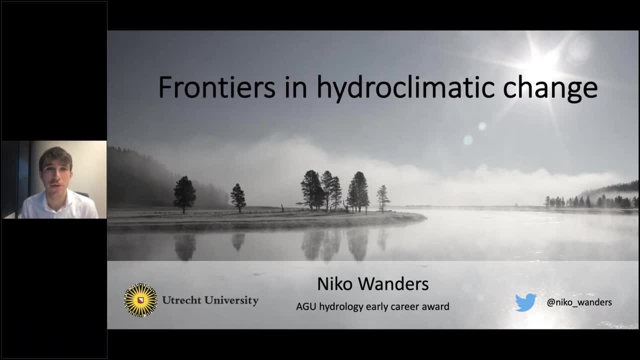 modelers win. uh, so yeah, first of all, we, in this case we actually validated with remote sensing data that was available, so we can actually look how the simulations look from. uh yeah, from a remote sensing point of view and, as you would say, an independent observation. and which community? 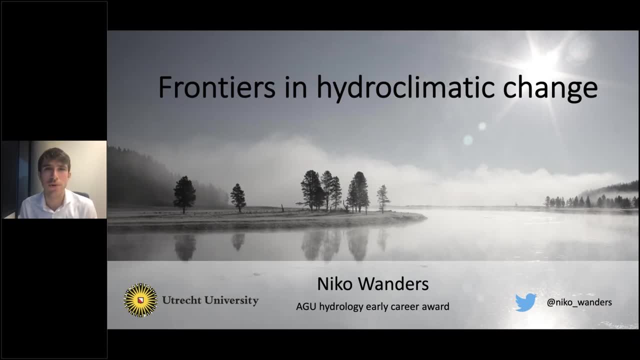 wins in that? that case it's a little bit more difficult, of course, for soil moisture, um, because we have, we have remotely sensed soil moisture, but that's only for the top five centimeters. uh, and the observations, that are points. so observations are: uh, yeah, i only have a very limited spatial. 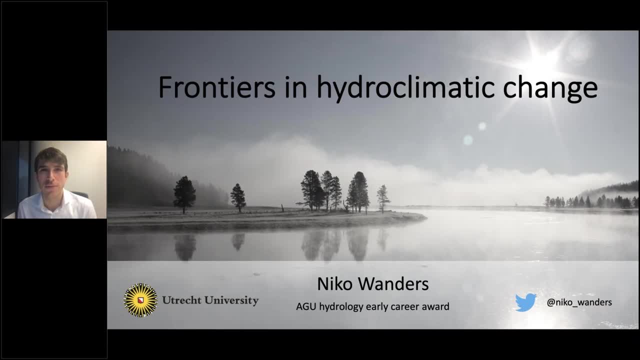 representativeness, so that's a little bit more tricky. in terms of groundwater, often they- or at least the model group we collaborated with- didn't have any groundwater interaction there. so that's that's something that we kind of win on, but i think you try to see with independent validation. 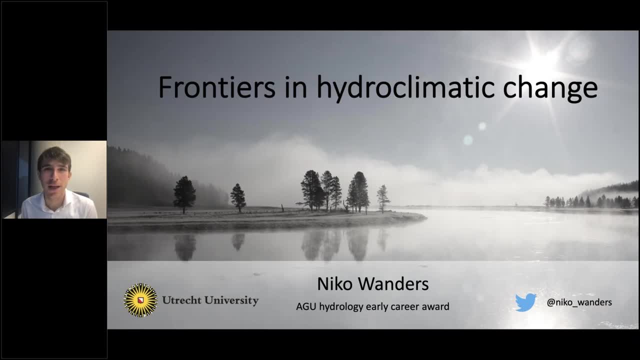 you know what's the best representation of the process, but then still, after coupling, things could get messed up. uh, of course, because coupling models doesn't always mean they're going to be better. but yeah, that's still up to uh, to that validation data set, to decide on how we can. 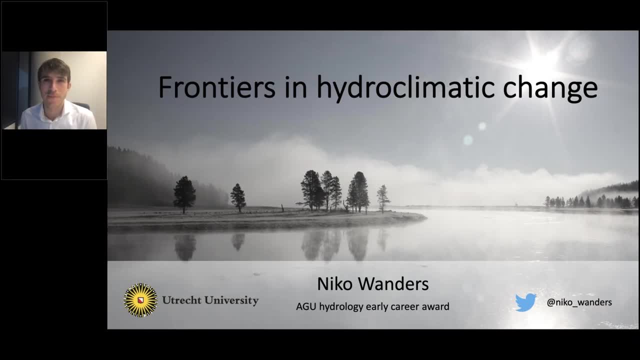 improve those, those couplings. okay, thank you very good. um, we have a question from- and i do apologize to begin with to my dutch colleague, wouter berghuis. uh, with the current generation of models that can incorporate so much detail, how do we quantify and communicate what part of the model outcome is robustly supported by data in theory and what part? 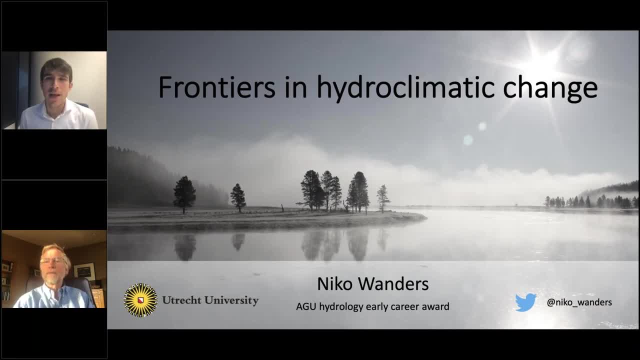 is still uncertain. yeah, i think that's one of the challenges, because if you go to these like 1k or step 1k grid cells, and it's very difficult to uh, to be able to validate in every point and be able to say i have full trust in all of all of it, especially if you start calibrating. 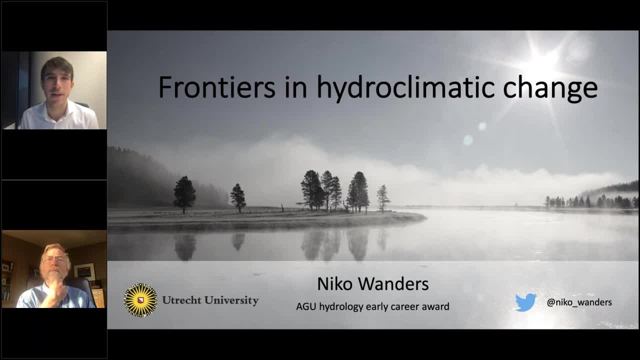 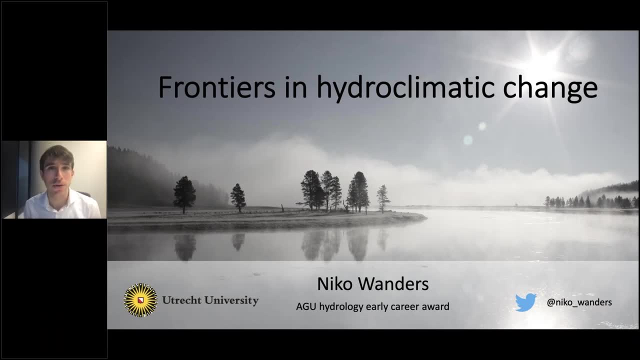 and in that sense i'm always in favor. uh, to not calibrate, it sounds a bit, but get the processes right. i mean, if we have the processes right and we get from an independent, independent observational source, we'll be able to tell: uh yeah, this, this mimics reality. uh, then you can have some faith. 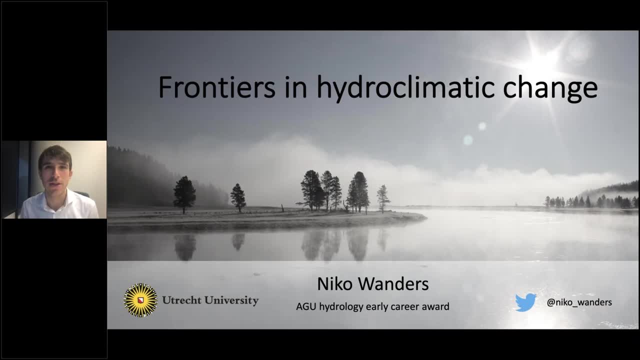 in that you can also do the same for other uh locations that you might not have any observations on. so for example, the, the graphs i showed uh from nate and the cheney his lai simulations. there's no calibration in that, in that process. so if you simulate lai and you get a picture, that is. 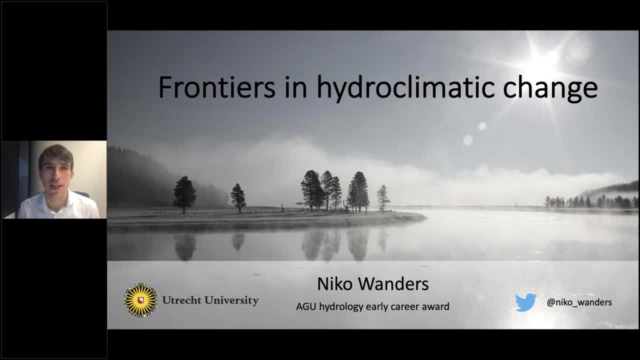 representative of a satellite image, then i think you can have confidence in that, that the modeling setup uh also performs well in other regions. but you always have to be aware of the caveats of our model. so for our global model, i know where i would trust and why i would trust it less. 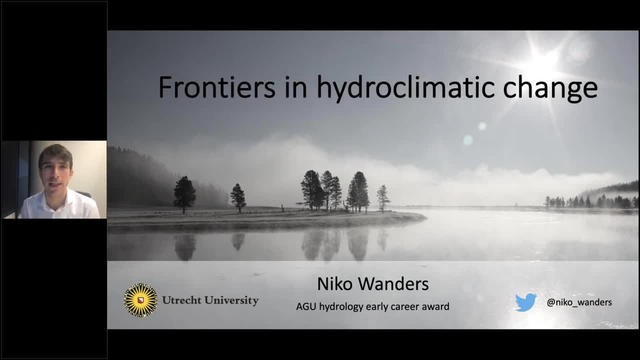 given our extensive validation we've done over the past- and i think that's also for the scientists to to, to be able to to capture that or give that information also to the user, whether that's a media journalist or whether that's a fellow scientist. i think you should be able to also. 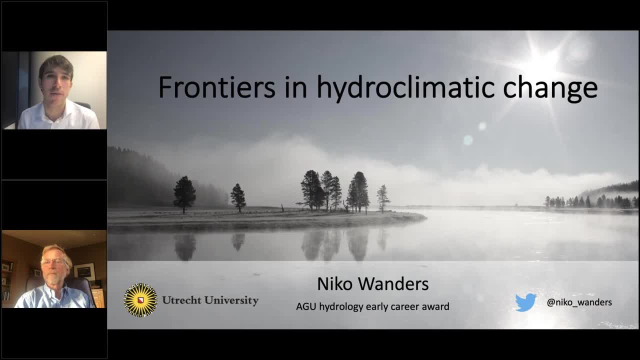 communicate your uncertainties there, where you trust the model and where you have little trust. i think that's. uh, yeah, that will be my answer, i guess. okay, thank you very good. uh, nico. this question comes from todd caldwell. i'm awesome to see these hyper resolution models. 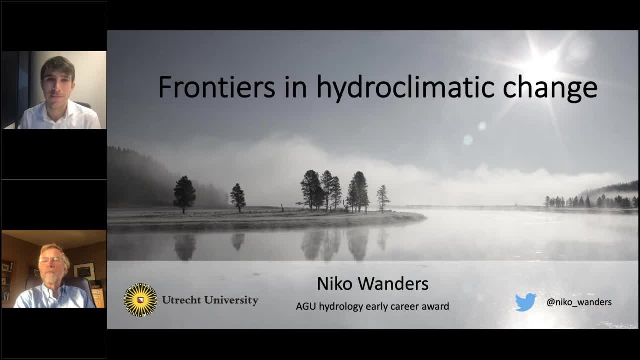 but, in your opinion, what data are still missing? what forms of data are missing to validate some of these models? in your opinion, what are the the biggest ones? yeah, i think. um, i think soil moisture is one that is really difficult than groundwater. uh, those two water sources we don't. 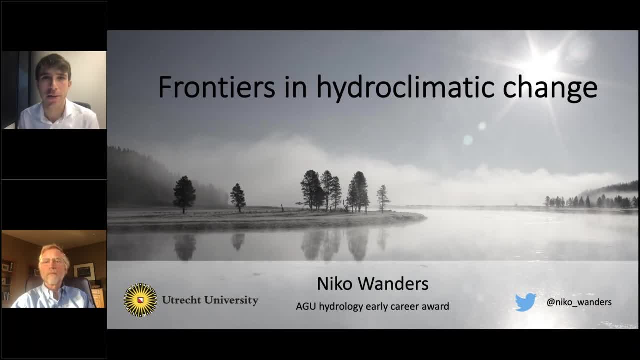 really see um. the spatial representativeness of the measurements that we have is limited and also the point measurement is sparse. so if you look at precipitation there are way more gauges. on discharge gives a kind of an integrated measure over catchment. of course, more discharge stations. 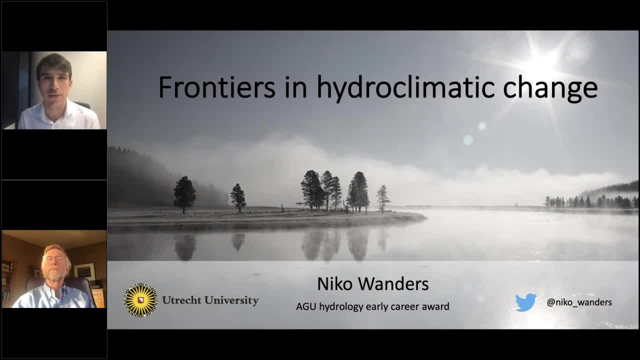 will be better, but for soil, moisture and groundwater it's very difficult because the spatial representativeness is limited and we don't have that many points uh to validate on. i think uh we both the united states and the netherlands- are fortunate in terms of groundwater measurements. 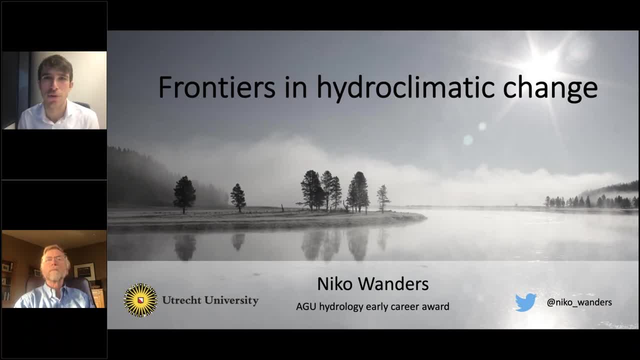 but if you go across the rest of the world, it's a little bit more challenging. and for soil moisture, i think, uh, yeah, that that's challenging around the world and um, but with the outcome of remotely sent soil moisture, i think we have gained, uh, some addition for grace, for example, for groundwater measurements. 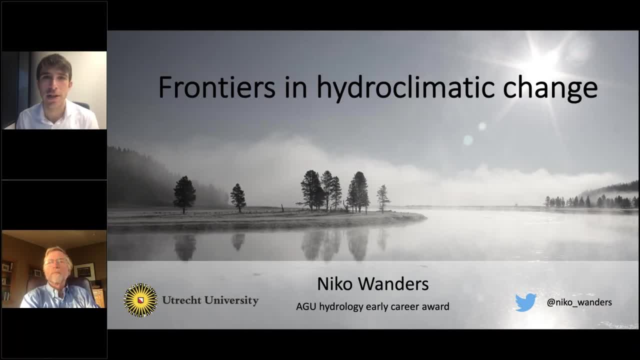 add something, but there's still quite a core spatial resolution. that definitely doesn't help to validate a model at 30 meters. okay, thank you. um, our next question comes from carol dahlin, and it's uh, ayniko. congrats for and thanks for the talk. 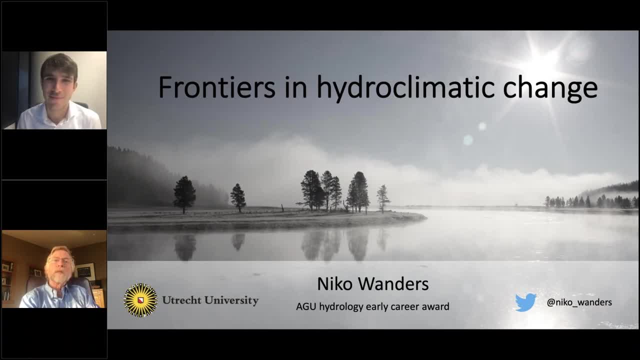 about human impact on drought. um is, is that right? the dams and reservoir intervention in your journal of hydrology paper leads to less drought? and if so, what about downstream water flow reduction? how is the drought defined in that case? yeah, so in general, on average it does. 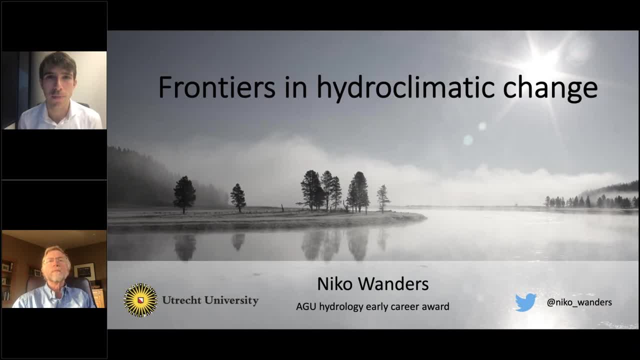 and that's because- but that's also assuming that you do the management properly. um, so of course, uh, you'll get additional evaporative losses, but by changing the flow distribution around the year you can actually gain more than you you lose in a sense. i must admit that for that paper it's, it's still. the evaluation is still on a basin level, or 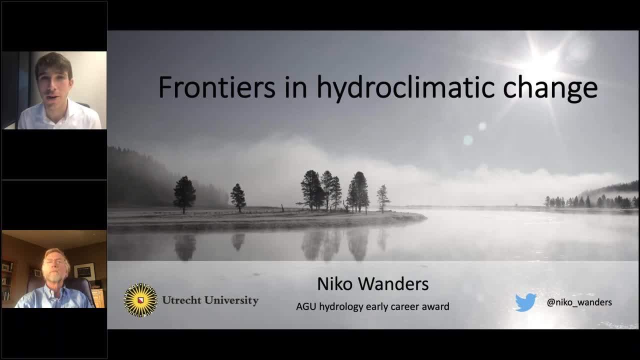 slightly closer than the downstream losses, which there are, and they are not negligible. they will be compensated by upstream gains, i would say so, um, yeah, i think i think that's also assuming that people do their management properly, and i i think we've seen a lot of 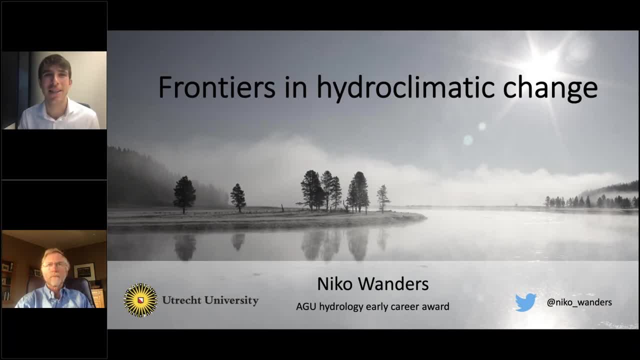 we've seen some nice- no, not nice, but we have some seen some real cases in where water management in reservoirs is challenging, especially with sentiments running high after droughts or before droughts. so i think that's still that's something that, yeah, is a limitation in that study okay. 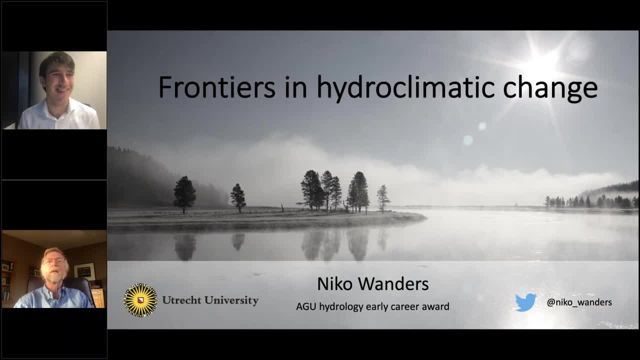 okay, and carol sends back a thank you. so thank you, carol. uh. the next question is: uh, suzanne groot, can you predict in which location or circumstances a high resolution model would perform better than a low resolution model in predicting drought? what are the criteria there? um, i would think that typically in areas with high uh heterogeneity, you 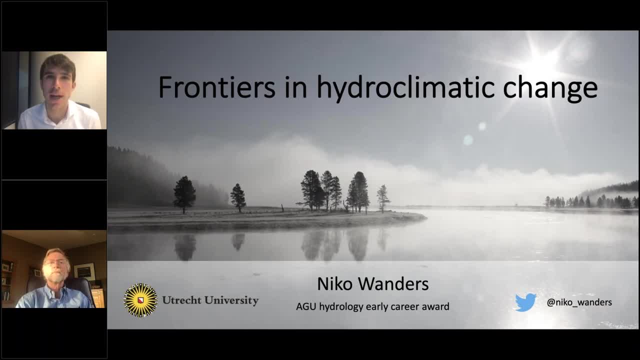 would probably have a more advantage of a high resolution model. we also saw that from foster studies. we saw that uh uh work at all. you saw that, like the, the changes in evaporation, if you look at a climate change scenario, you see some very uh impressive uh, evaporative changes and that's uh, it's often. 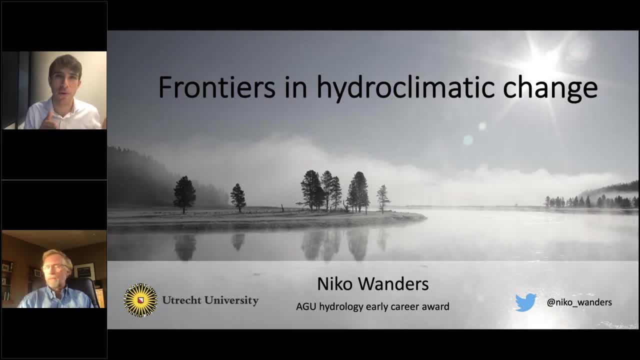 at least, uh, also combining it with the things we see in the cheney coupled work. um, there you can. i can hypothesize that it's either close to streams or very far from streams, so that kind of slow uh, or that that high heterogeneity within it in the landscape. 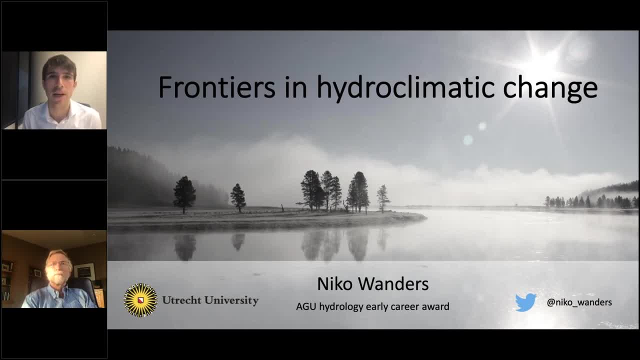 would actually also make different changes in terms of how the process is dominant at different locations. so i think, uh, if you have that, that higher heterogeneity, simultaneous regions- uh, let's think about the rockies or something. um, yeah, there, i think you would gain a lot. the difficulty there, of course, is the 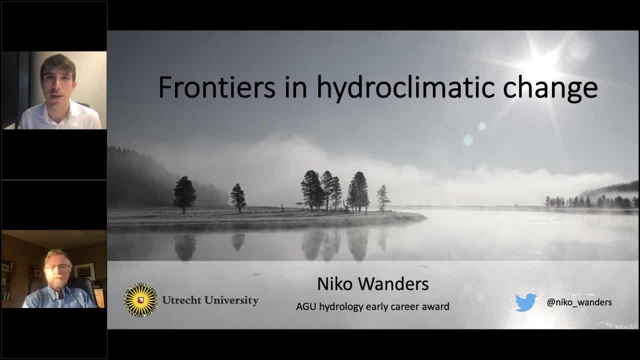 parameterization, uh, which would suffer from this high heterogeneity and and the lack of input data we might have there. so that's, that's a downside, um, but yeah, i think that's where, in the end, we would gain most. also, if you look at precipitation gradients, and- but we don't have the data on that. 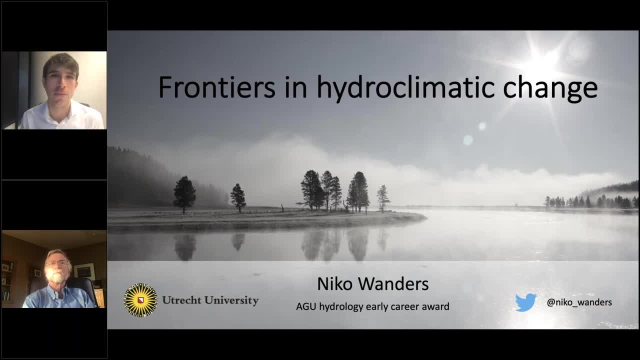 and- and, in fact, you know the only way to explain that is to say that it is uh, uh, there's a very high, um, a very high level of spatial resolution. that's the ground level of spatial resolution, um, but it's also uh, it's also not the case as well, uh, and so it can be. 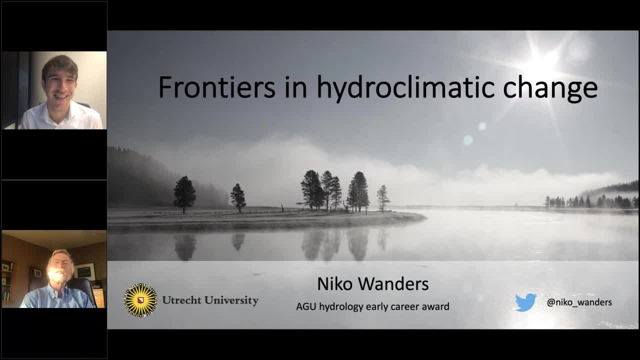 interpreted as a very unoriginal device, and so that's there's no, there's no general disagreement on why it's possible to just do a very high level of spatial resolution with like a 3D gradients and and runoff process on very steep slopes that cannot be captured by the large scale. 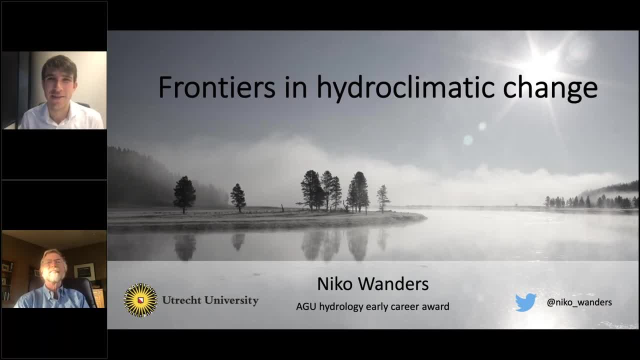 projections of drought intensity: Uncertain. That's a couple of uncertainties. Yeah, I think it's still our hydrological modeling chain. So I think the GCMs, or the forcing data, is there, or at least they show a larger consistency than the representation we have. 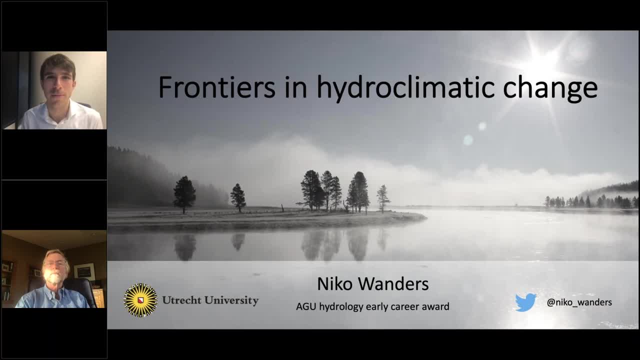 in our hydrological models at the moment. Also, looking at some of the papers, for example by Prudhomme and Lieke's paper- Lieke Mels's paper as well- they also confirmed this And I think how we incorporate the processes. 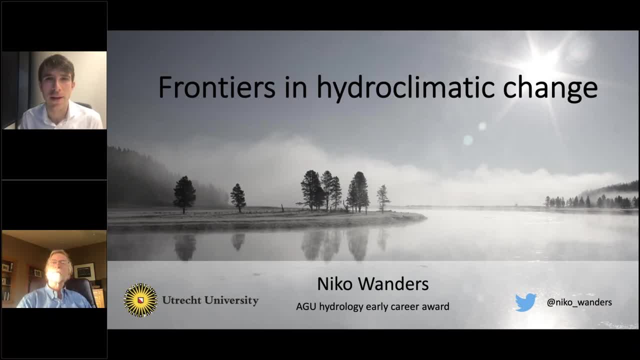 and what resolution, what detail, and that all matters towards how the future projections look. We've recently done a project with UFZ, the Edge project, and we had four hydrological models and already the differences were noticeable, while the GCM data was more or less in the similar direction. 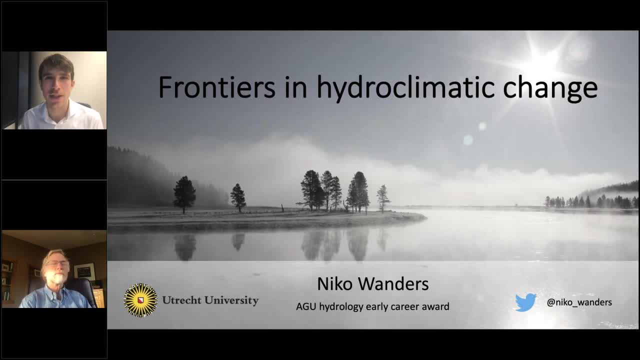 So I think as a hydrological community that's still a challenge. I'm not sure. I'm not saying we have to always use one model that's the best model, or always take an ensemble, but be aware of the different results that you will get with the different models. 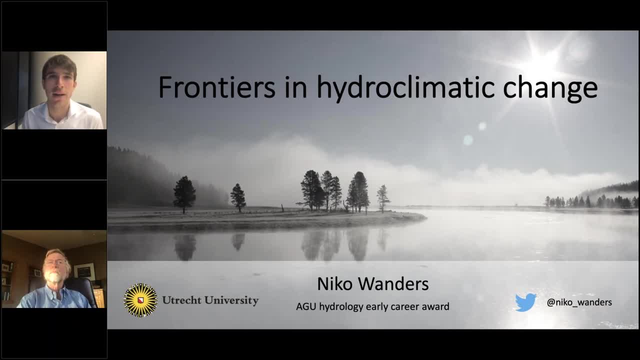 especially when you want to draw very large conclusions. For example, is human water use and human water feedbacks? are they included in your model? That does make a difference. And if you have a natural system that actually limits us, of course, then in a sense, the climate projections, you can do. 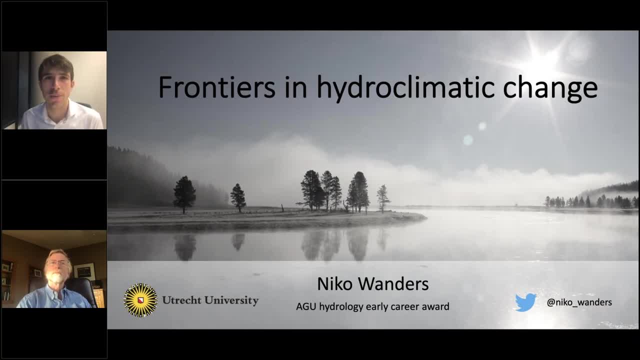 or at least the confidence you can have to say this is what's gonna happen. Okay, thanks. Perhaps suggesting another round of model inter-comparison is needed. There are already some, I know. I know, yeah, but it's serious, yes. 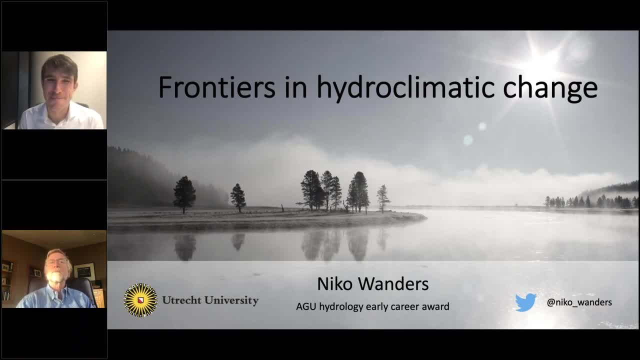 All right, So a good question here. thank you, Mark. A good question from Sally Rangecroft, and this is a tough one. How do you best overcome the challenges of communicating uncertainties related to your modeling to the general public? 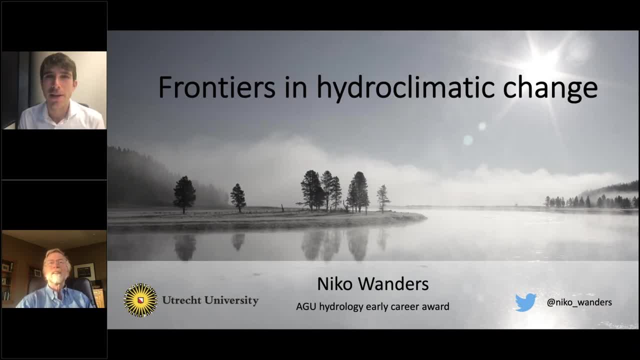 Yeah, that's a very tough one, because what I typically try to do is, or what I try to show is like what the uncertainty looks like, And if you say, for example, a drought is, or at least the chance of drought, double. 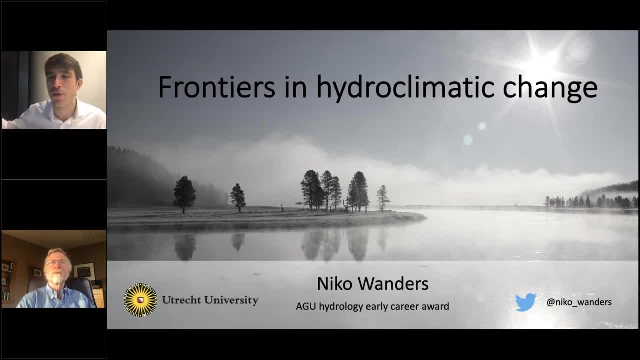 if you want to say that, then I often say within a time range of between 30 and 50 years from now, not saying it's gonna be 40 years from now, but giving an indication of the range And I think most people can actually. 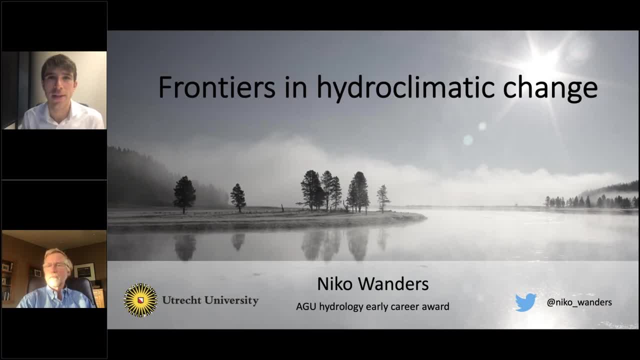 yeah, when you give such a lecture and they understand that there's uncertainty on these things, And I think it's also more convincing message if you actually give them the full message rather than just say, within 40 years, droughts chances are gonna be doubled. 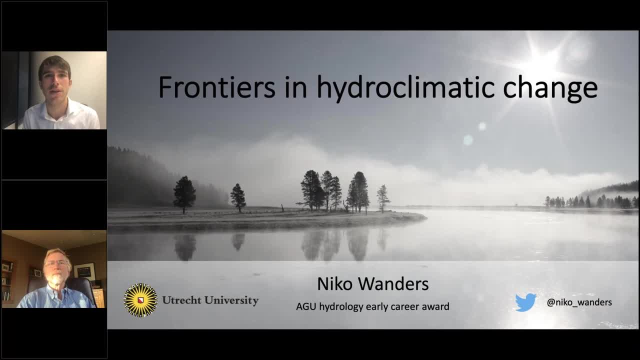 So I think by including that and also showing them the graphs and the uncertainties, I think that helps. For some things we can be more certain than for others. we shouldn't make any comments on things we don't know for sure, But I think by showing it and also children 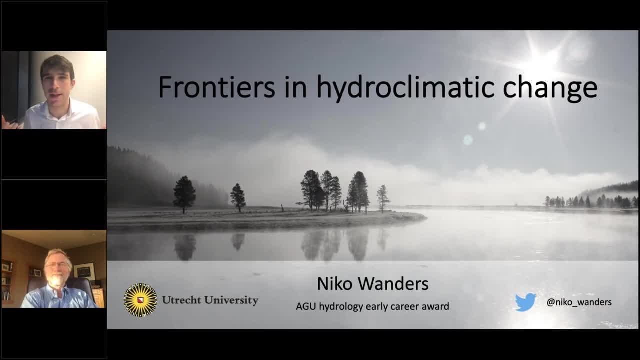 I mean they understand how you roll a dice, for example, how it can. the outcome is never certain, but you have an average way it's gonna look like the average will be three and a half, but it can be a six one time and one the other time. 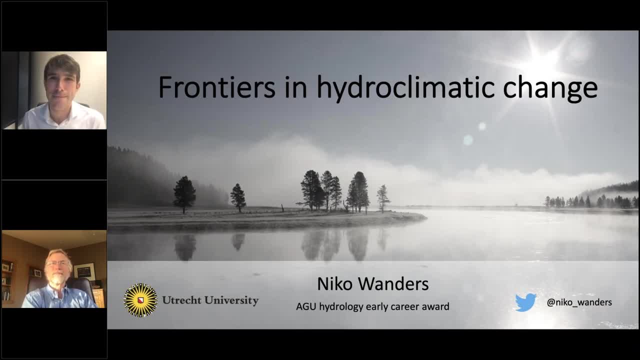 So, and they understand that as well. So, yeah, Okay, thank you. I think that would make a great, a great town hall or panel discussion at the next, the 2021 AGU meeting to talk about experiences of kind of communicating. 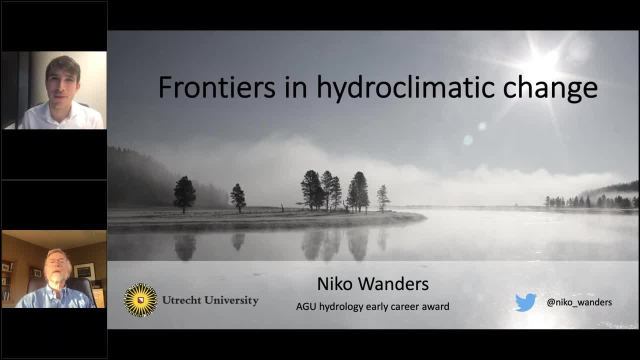 these uncertainties. All right, our last question comes from Remco Aulenhout- excuse me- and Nico, which is who won the bike climb at the AGU 2019 meeting? Apparently, it wasn't Remco. No, he didn't join. 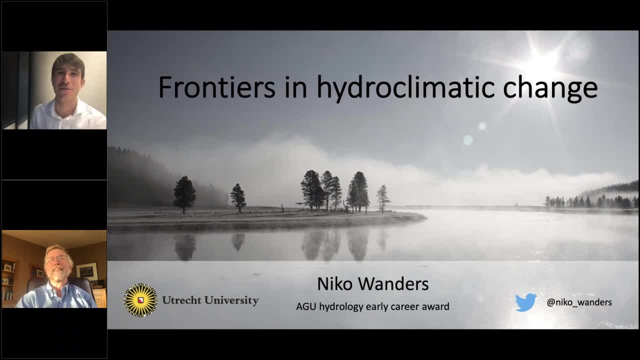 So that's a bit. you know, I always try to get out with some of my collaborators to go the day before AGU, So I will not name any names, but it was a nice- let's put it's always a very nice ride. 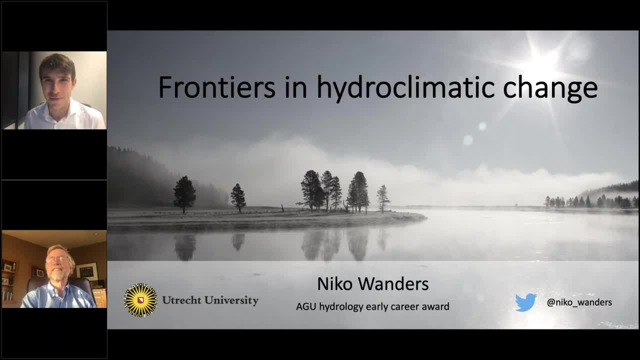 that we can exchange ideas and have some fun. I think that's the most important thing that we can have- and the friends that you get from those science and AGU full meeting gatherings. So next time Remco can join if he wants to. 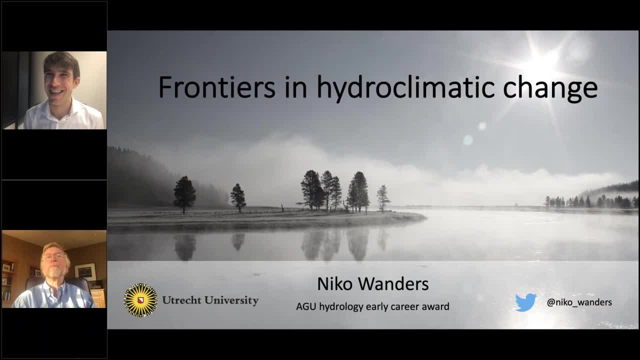 Okay, next time I'll join It's in New Orleans, so it won't be much of a climb. Very good, All right. Well, thank you, Remco replied diplomatic answer. So thank you, Nico, from the audience. 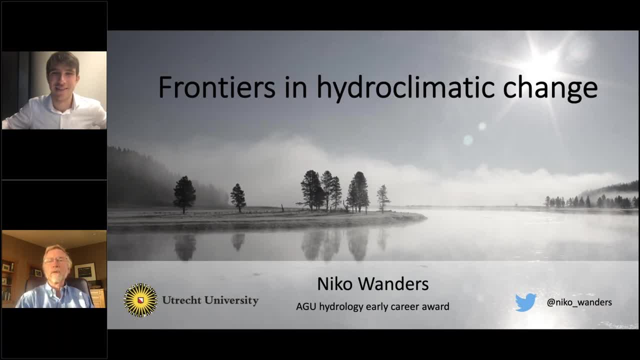 If you will, let's give Nico a rousing round of applause. Wonderful talk, Nico. Thank you very much, Much appreciated and stimulating, And we look forward to seeing you virtually at the AGU meeting and thank you. Thanks, Scott, thanks. 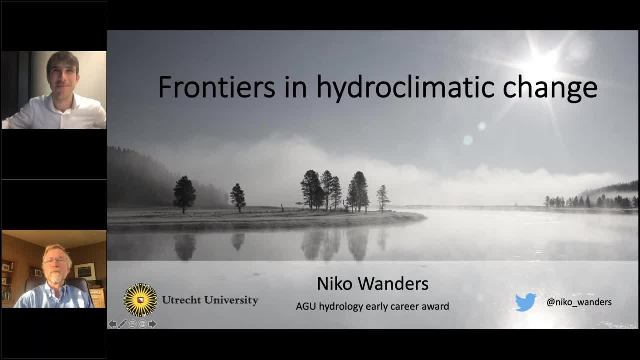 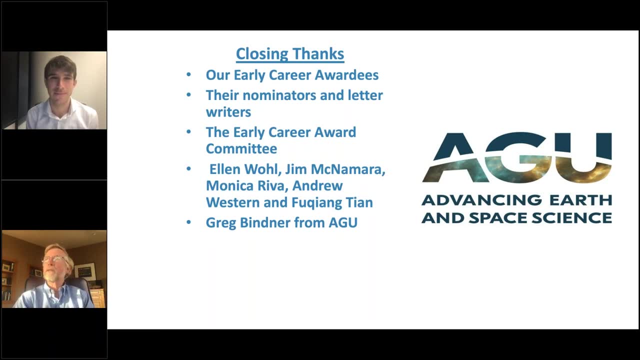 Very good. And, Nico, if you can just put your hand up, You just popped to your next slide. I've got a couple of things to say. I just wanna thank everyone. So this concludes our three parts early career awardee lectures in November. 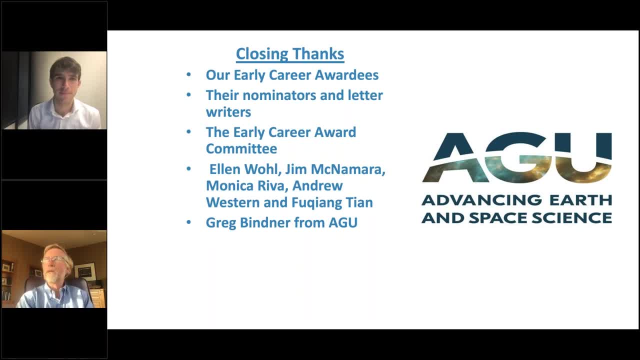 I think they're really successful. I think we can do this again each year. I hope so, And I hope I'd love to hear feedback from all of you who have been listening over these last couple of Friday mornings. Thanks to all the folks who nominated. 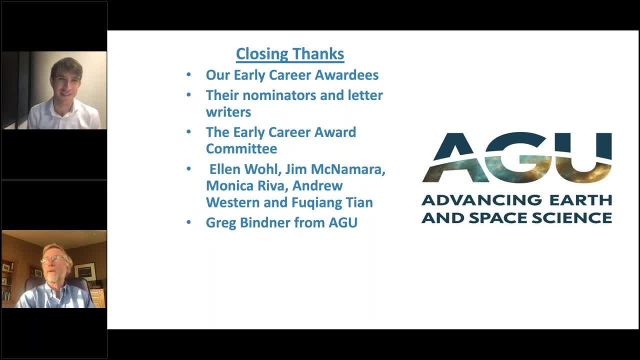 our early career awardees And all of the early career awardees. We had quite a big, quite a large pool this year. So thank you very much And all the letter writers. I also wanna thank the early career award committee. 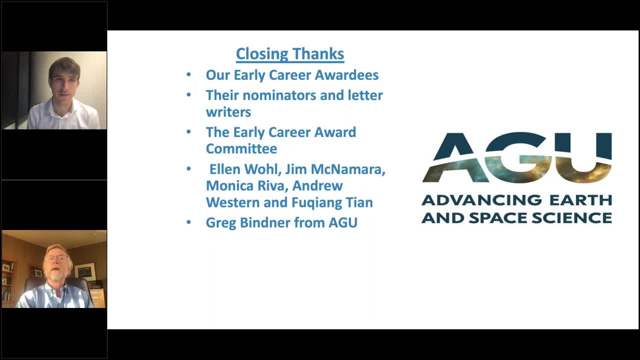 which is chaired by this year, was chaired by Ellen Wall and had members Jim McNamara, Monica Riva, Andrew Western and Phuc Nguyen Tien. So thank you very much, And also I just wanna thank Greg Bindner from the AGU. 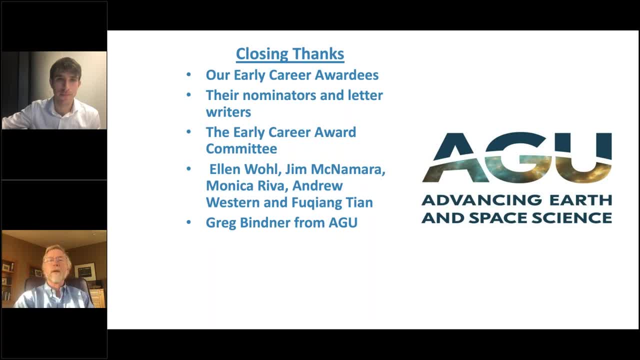 who's been in the background here. None of you have heard him too much. He's been making sure that this webinar moves smoothly through, So very much appreciated to him And I think we've had really ease and good work through this. 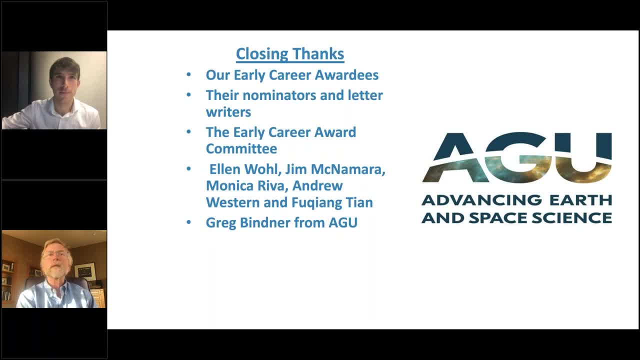 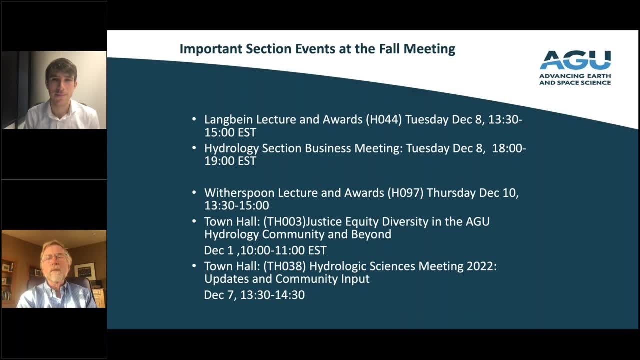 So thank you, Greg and all AGU. Nico, next slide, if you would. There we go. Okay, a couple of things just to remind everybody what's going on. I know it's a confusing meeting and it's a challenging meeting. 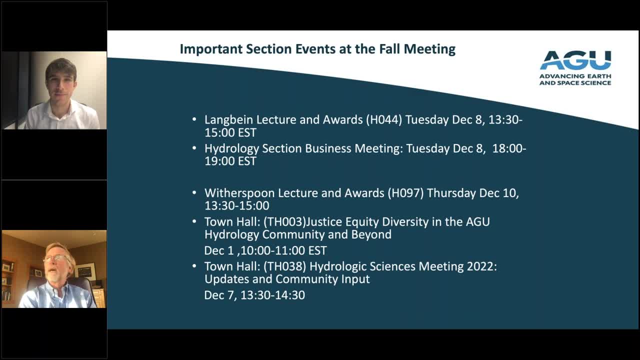 First off, before we get into what's happening at the meeting, I sent out a note late yesterday because I got heads up from AGU That for those of you who are worried about uploading your presentation, which was due today or is due today, 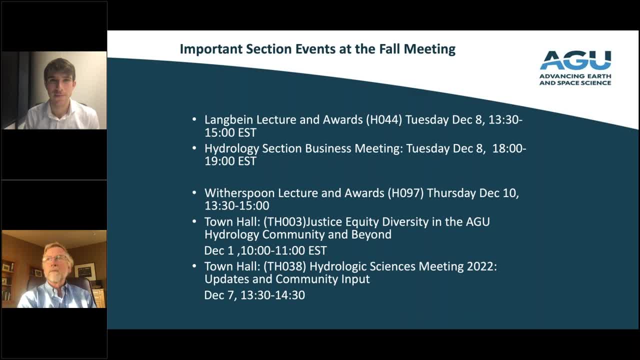 they're giving everyone a grace period until Monday, this coming Monday- And I'm not gonna say what time it is because I can't remember the time, but it's in your email. I sent it out. It's also on the hydrology website. 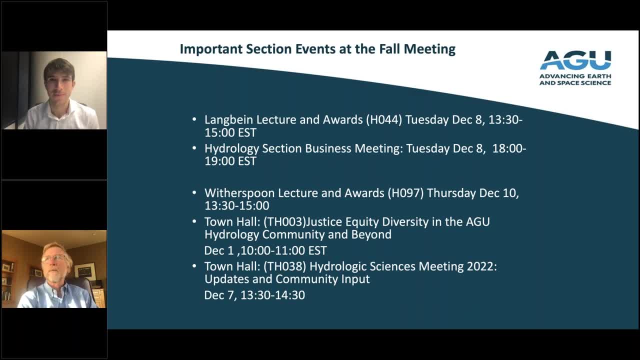 So you do have a little bit of time. over the weekend They realized people were getting a bit panicked, and I'm sure many of you may be getting a bit panicked. So calm down, Everything will be fine. A couple of the important things for the meeting. 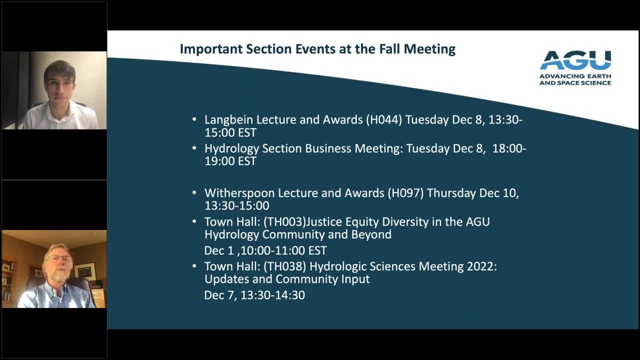 So first off let's go to the. we're trying to keep our events that we do when we're in person, kind of on the same timeframes, so that we keep some traditions and we don't confuse you too much. Still will be confusing, but we'll do the best we can. 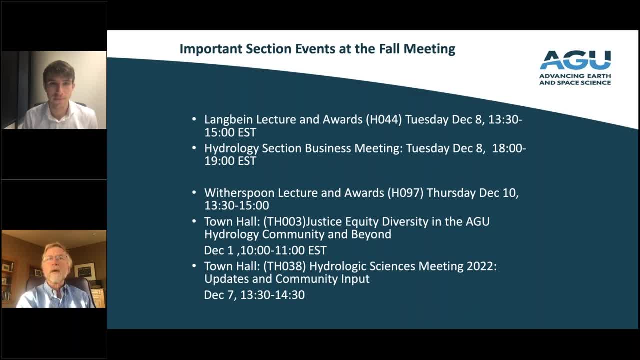 So as normal, our Langbein lecture will be on Tuesday, and that's December 8th, And that is from 13 to 1500 Eastern Standard Time, So kind of afternoon Eastern time, early evening European time, And we will also do part of our awards. 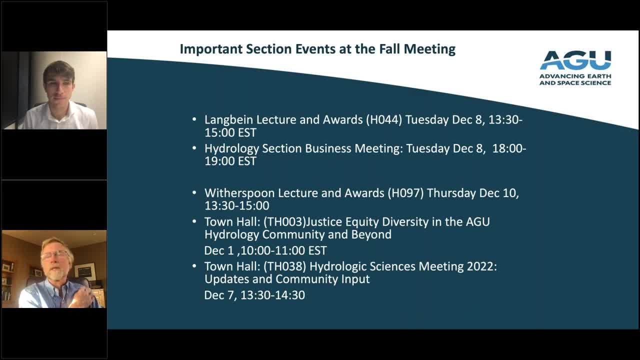 during that Langbein lecture, because we don't have quite as much time as we normally do. We're going to split the awards. Our Witherspoon lecture. the other lecture is also on Thursday. It normally is on Thursday, same time. 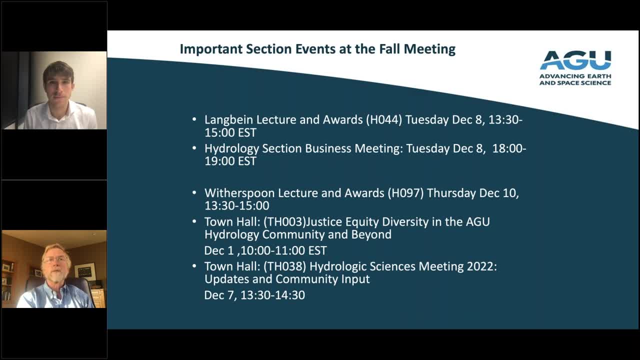 And we will. that's where we'll celebrate, actually, our early career awardees during the Witherspoon lecture. The lectures will be recorded but there'll be live question and answers after each of the lectures. The Hydrology Section business meeting is on its normal date and time. 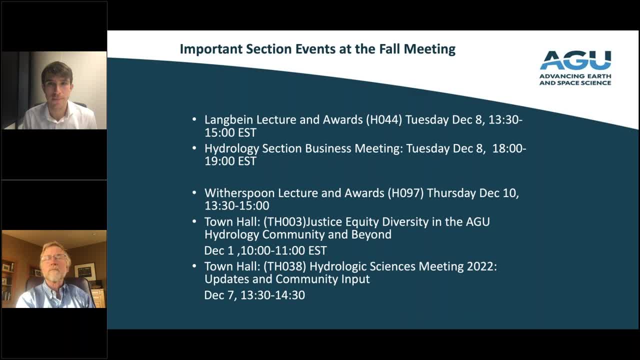 Tuesday, December 8th, roughly dinner time, East Coast time, So it's okay to bring your beverage to the business meeting. That lasts about an hour. I do encourage all of you to tune into that. Basically, it's an update of what the section is doing. 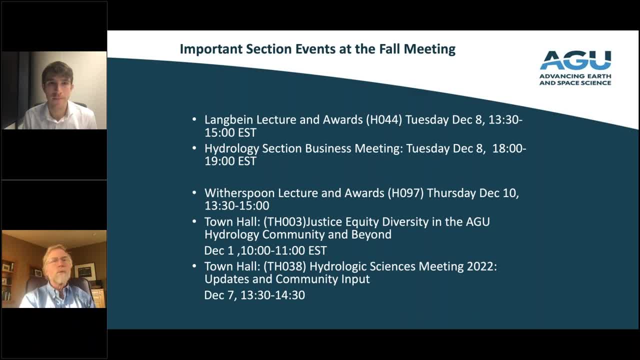 what the section has done over the past year and where we're going for the next year. You'll get to introduce, we'll get to see the new section office, We'll get to see the new section officers, et cetera. 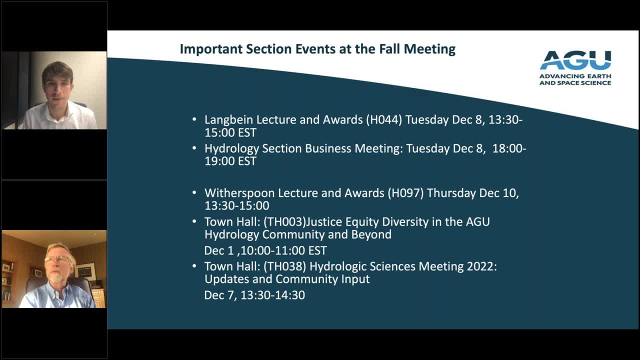 and hear from Kwasi, from Water Resources Research, from our student section and from our OSPA award winners. All right, so those are the key things. as far as our normal things, Town halls, two town halls I want to call your attention to. 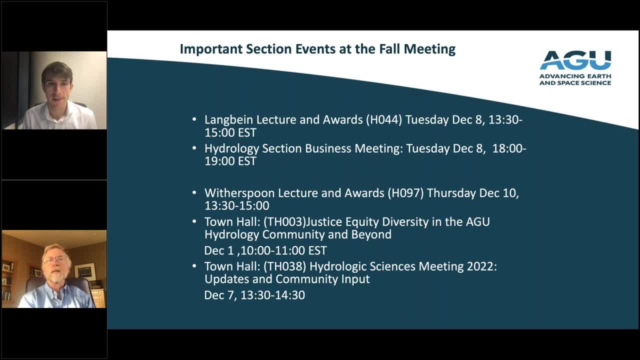 One is early in the AGU meeting December 1st and that's a town hall put on by our student section to talk about what the section is doing and can do and hear from you about justice, equity and justice. Thank you. 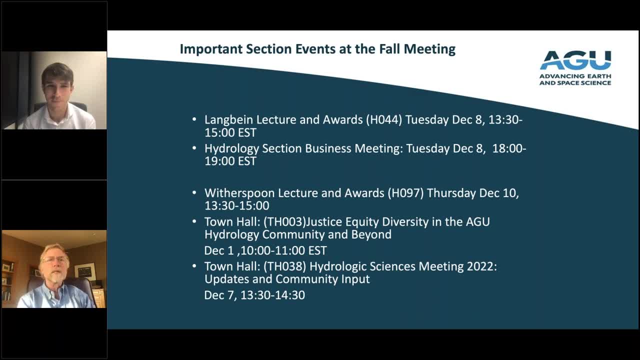 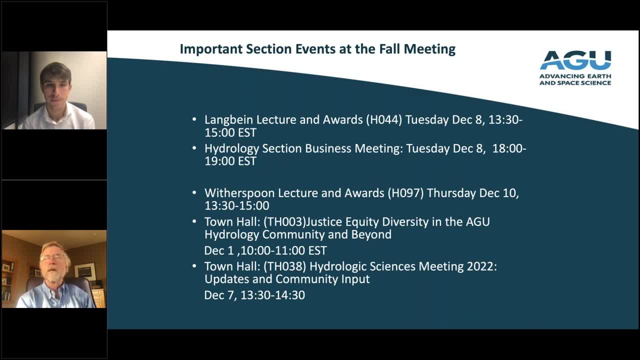 the meeting that will be held in 2022, joint with Kwasi. So we'll give you some updates there and then we want to get some community input back on those. Let's see what other things do I need to tell you? 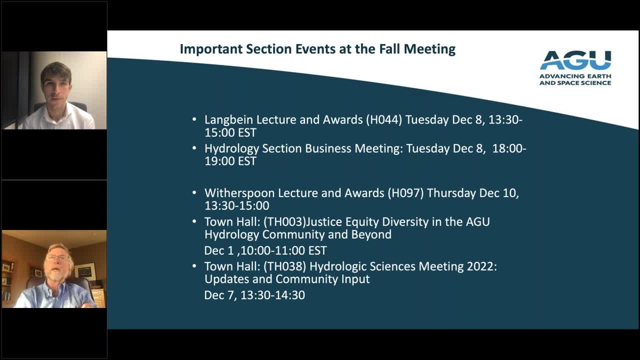 Ah, one last thing thing which is keep an eye out, We're working on having, during what would normally be the cocktail hour at the fall meeting, we're hoping to have kind of meet and greets for the various section volunteer groups. So we'll have a WRR meet and greet one evening. meet and greet your technical.